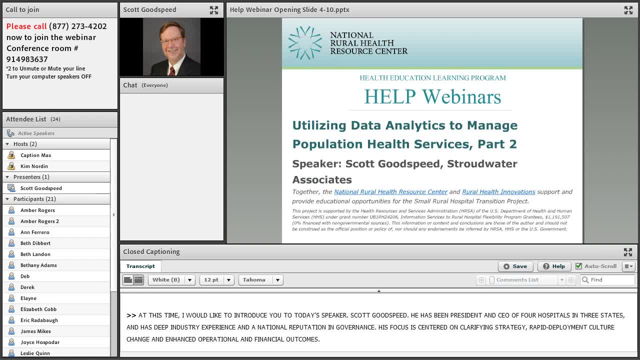 rapid deployment, culture change and enhanced operational financial outcomes. A nationally recognized speaker, Scott has authored and delivered over 500 presentations to various professional associations and healthcare organizations on topics such as strategic planning, health industry trends, 21st century governance, constructive cultures and the 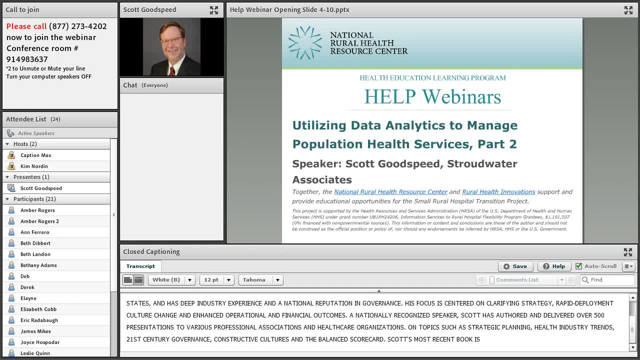 balance scorecard. Scott's most recent book is titled Community Stewardship: Applying the Five Principles of Contemporary Governance. He has recently written two articles on population health and reducing waste Using comparative analytics. In addition, he is conducting research on organization and board culture, which will culminate in a book with a current working title: The Culture. 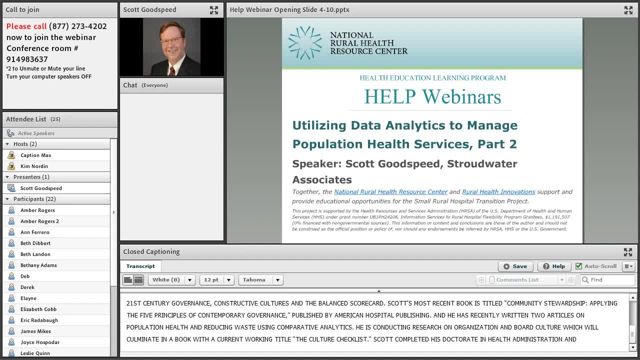 Checklist. Scott completed his doctorate in health administration and leadership with a dissertation entitled The Balance Scorecard: Translating Strategy into Action. He received his master's degree in hospital administration from the University of Minnesota, where he was recognized for his academic achievement. 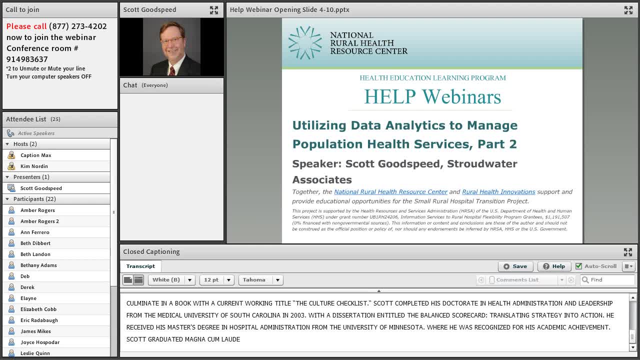 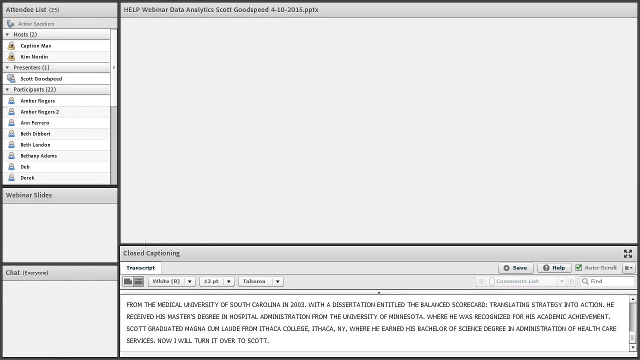 Scott graduated majoring in magna cum laude from Ithaca College in Ithaca, New York, where he earned his bachelor of science degree in administration of healthcare services. Now I will turn it over to Scott. Scott, are you there? 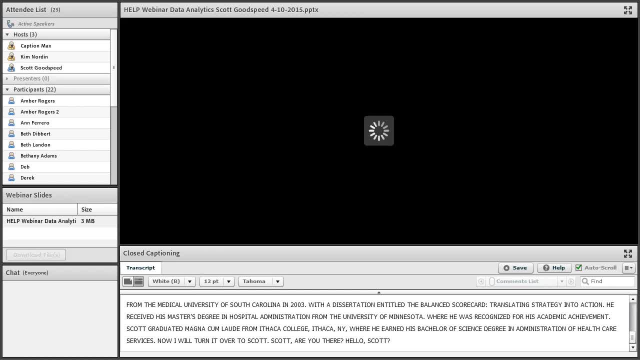 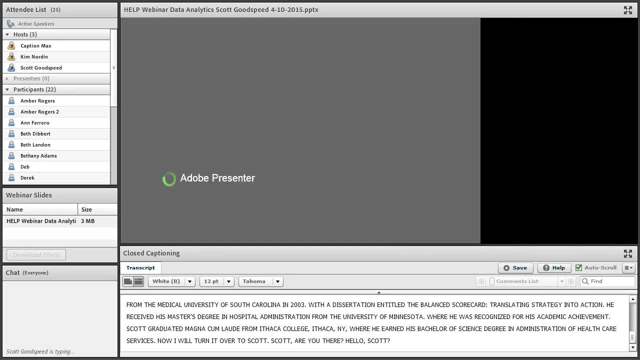 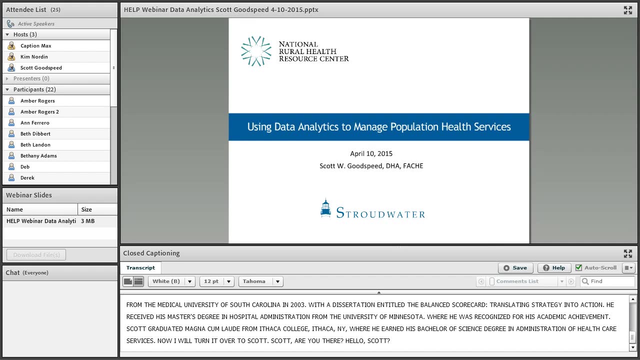 Hello Scott, I'm here. Hello Scott. Oh, You're good for the job. Mmm, yes, And you look tired. I won't tell you. Oh, One moment, while I locate Scott. Scott, if you're on the line, please press star 2 to unmute your line. 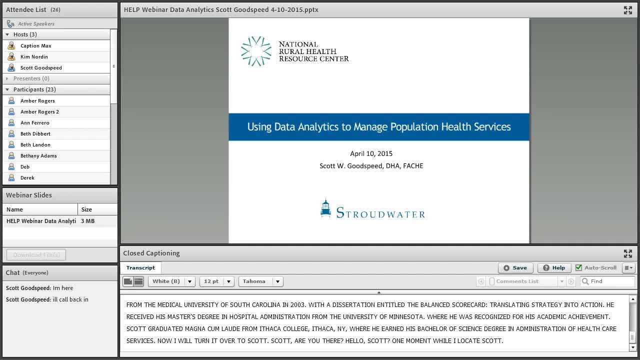 Scott, are you there? you all right, it looks like Scott is having a little trouble connecting, but he will be calling in and should be here in just one moment. thank you for being patient, everyone. Scott, are you there? can you hear me? Hi, I can hear you. 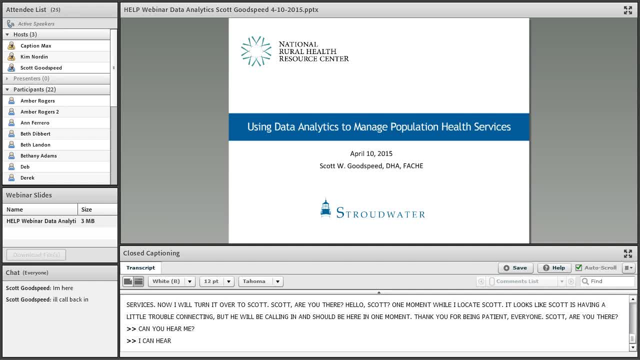 I'm not sure what happened last time, but let me get going. I call back in. all right, wonderful. sorry about that everybody, but I wanted to thank Kim and Leslie and Bethany and Terry Hill at the National Rural Health Resource Center. for those of you who are, 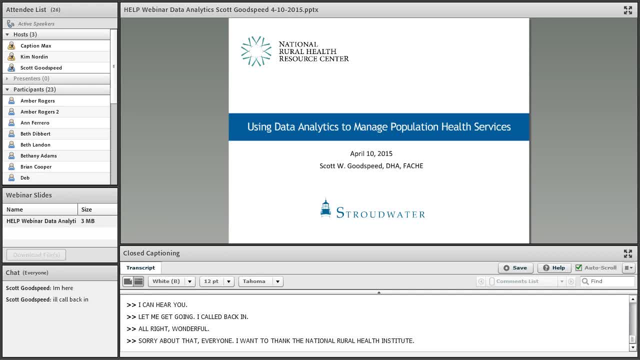 who are on the call. Wednesday we talked about how we're moving from the state of the city, from fee-for-service, to population health, and we talked a little bit about. population health is defined as health outcomes of a group of individuals. it could be by age or disease entity. we also talked about 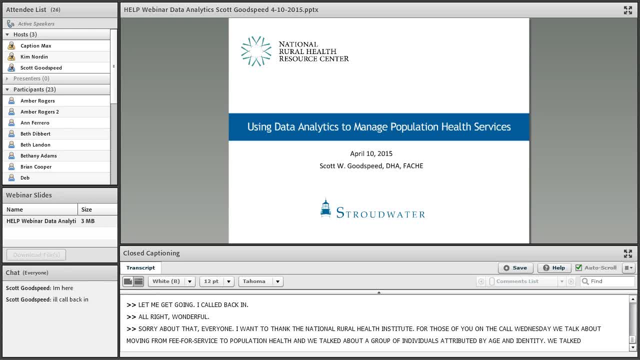 understanding a new language and at a minimum we need to understand our service area. as it relates to a 10-year insurance projection and when we get done, the call any of you that want that for your organization, the service area more than happy to to do that. just as a reminder, we also talked about one. 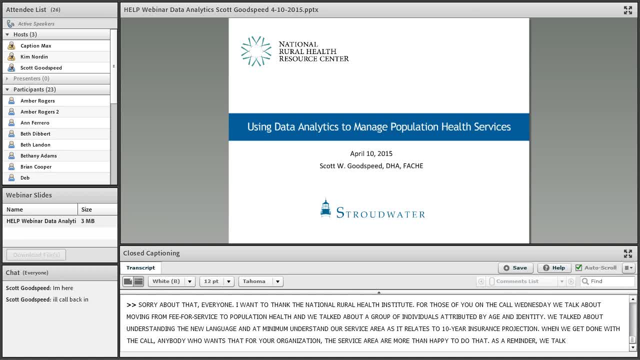 percent of the population with the highest spending accounts for about 23% of the total population, and that's the top five percent of the population, is responsible for almost half of the spending and that comes from the Kaiser Foundation. I don't know if there's anybody on from New Jersey, but I'm going. 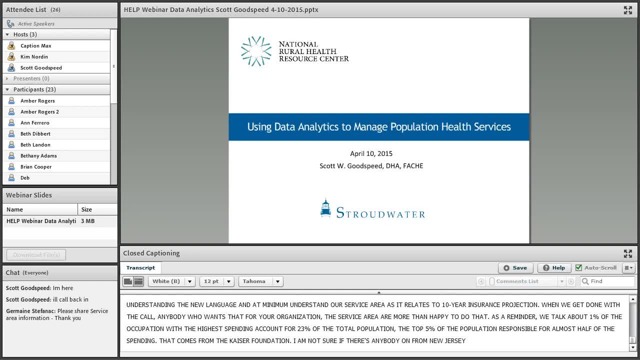 to talk about the Camden experience, and when you hear a little bit about the Camden experience and health care expenditures, it's going to mirror the Kaiser Foundation experience, if you, if you will. so the other thing I just want to mention is we did get a question from a physician at the end of the last call. we just didn't. 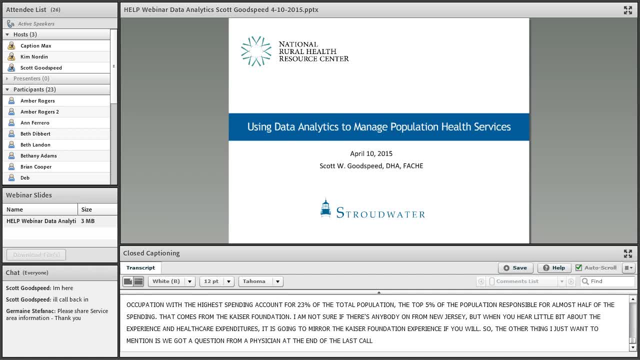 have time to answer, but it's an interesting question because it really relates to population health and relative value units and the and the question was: could you provide some guidance on how to start a new population based management system from an RVU physician perspective? so so what I basically said to him is: relative value units as a 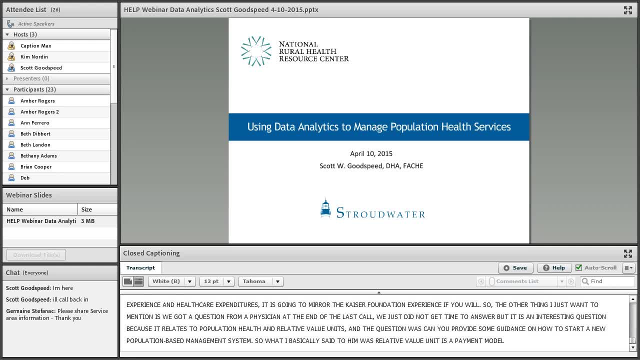 payment model has been dropped for a number of primary care providers, and the best example I know of is Fairview Health Services in Minneapolis in 2007. in 2011, the health system dropped their relative value units as a payment model for primary care providers and established a comprehensive 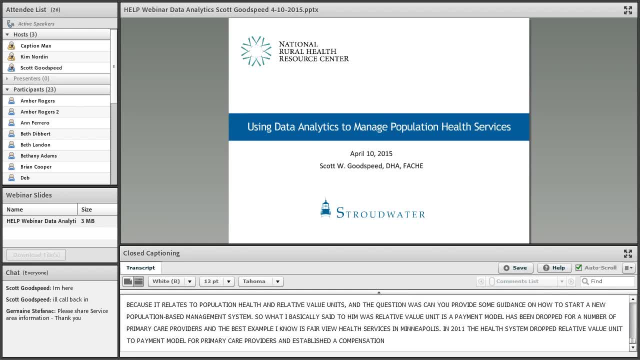 compensation framework that ties 40% of the physicians payment quality metrics and population health and 10% to patient satisfaction. so we didn't spend a lot of time talking about physicians or providers, but but there's a way of tying in incentives on the provider side to population health. so today we're going 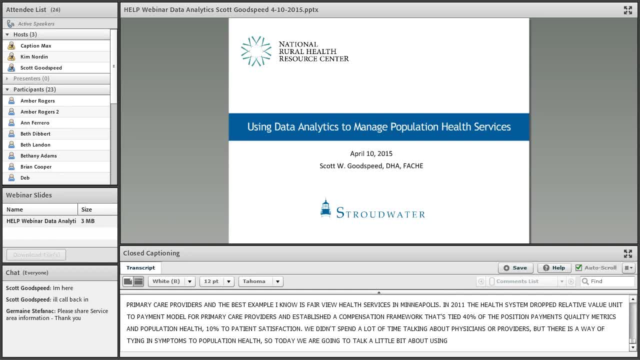 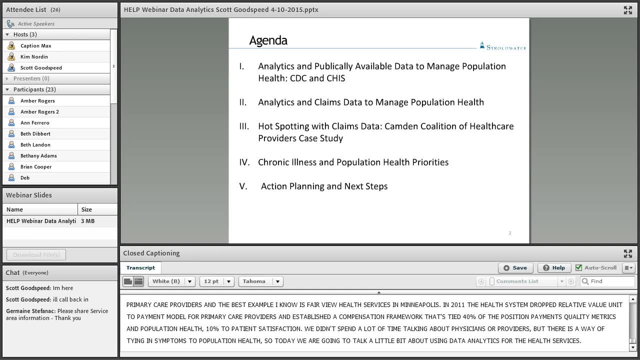 to talk a little bit about using data analytics to manage population health services, and we're going to talk about some publicly available data. so sometime in the next week I'm going to ask you all to jump on the CDC website. I'm going to show you some screenshots- the pretty interesting thing about this website and 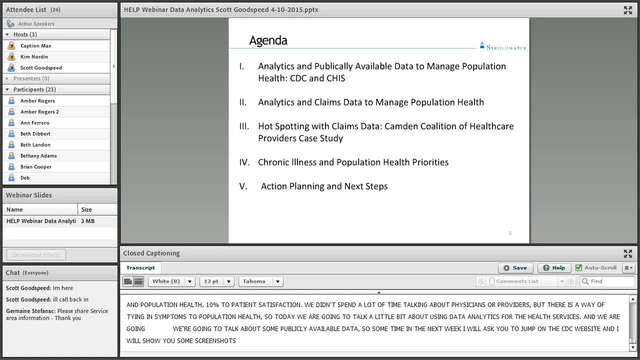 what they pull together. it's been publicly available since March 10th, so just about a month ago, 2015. we're going to talk about how you can use analytics and claims data to better manage population health. and we're going to talk about how you can use analytics and claims data to better manage population health. 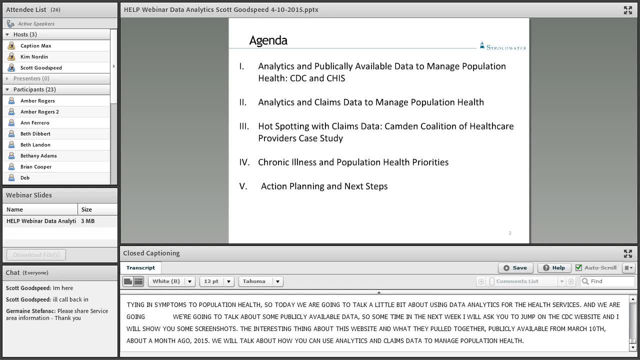 and we're going to talk about how you can use analytics and claims data to better manage population health. I'm going to give you the experience of the Camden coalition of healthcare providers as a case study. a group of providers, community members, school systems, social service agencies, other community agencies- came together in 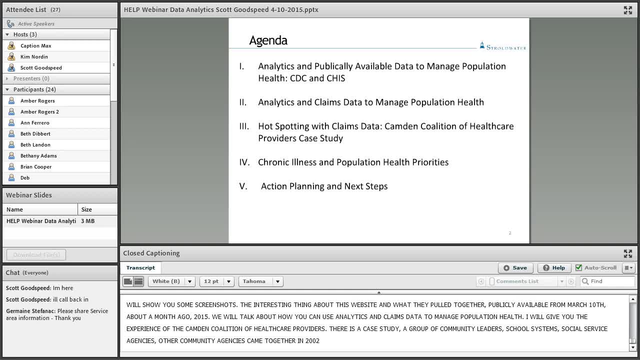 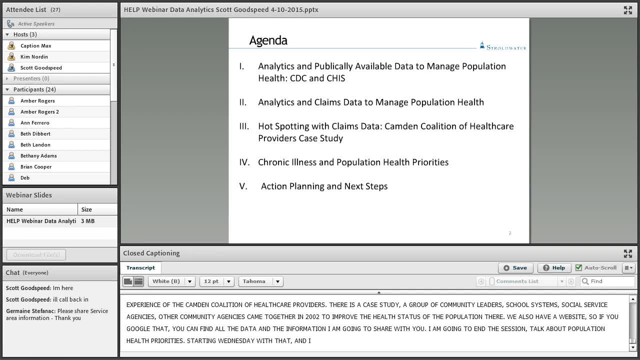 the website. so if you google that, you can find all of the data that's available on. We kind of started Wednesday with that and then I'm going to suggest some action planning and next steps, And the other thing that I'll offer next week is any of you that want a 20-minute private conversation, you know. 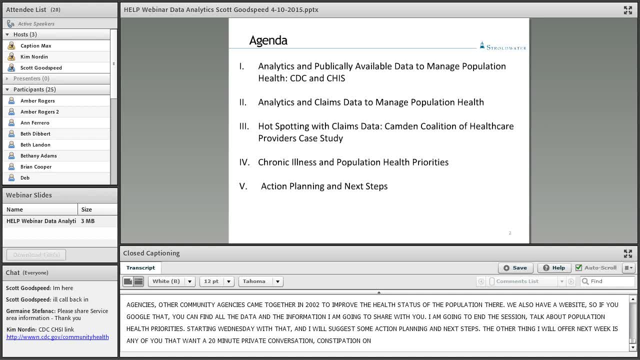 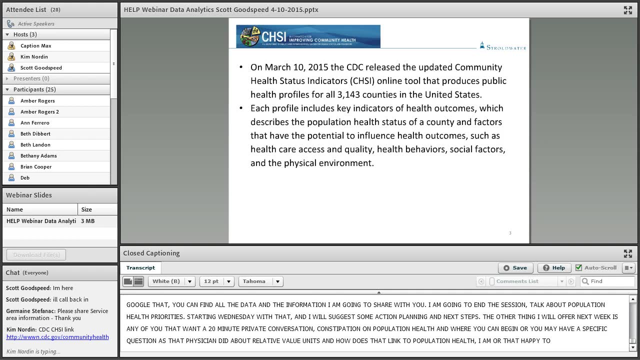 consultation on population health and where you can begin. or you may have a specific question, as that physician did, about relative value units and how does that link to population health. I'm more than happy to do that and provide that. So this is the – I'll share with you the website. 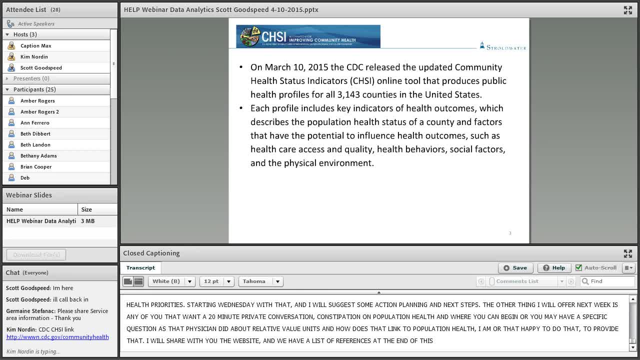 and we've got a list of references at the end of this presentation. But exactly a month ago, the Centers for Disease Control released their updated community health status indicators, what they call the CHSI. It's an online tool that produces public health profiles. 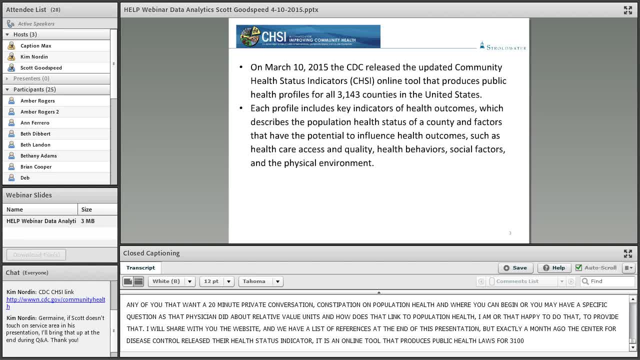 for over 3,100 counties in the United States, And if you're going to start with publicly available data, I suggest you begin here. So each of the profiles includes indicators, as it relates to health outcomes, that describe the population health status of the county where you're located. 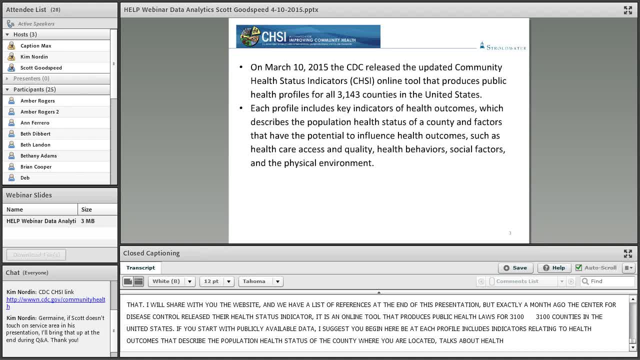 talks about health care access, quality health behaviors, some of the social factors as well as the physical environment, And then you can go ahead and check that out. And then you can go ahead and check that out. And then you can go ahead and check that out. 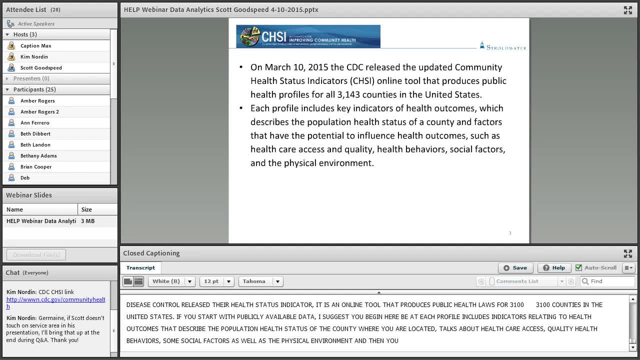 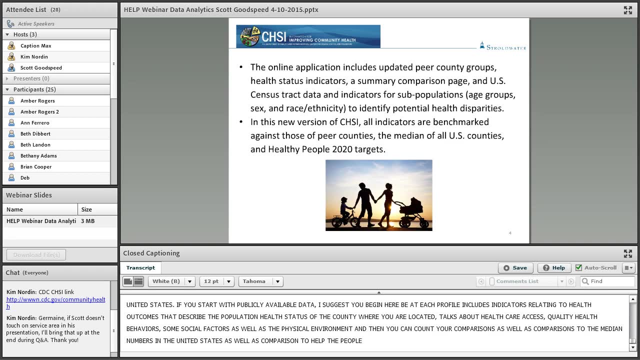 can get county peer comparisons, as well as comparisons to the median numbers in the United States, as well as comparisons to healthy people 2020. so this is a this is a great starting place and this is a free. it's a free online tool. as I mentioned, you can- you can look at peer County subgroups. you can look at it by: 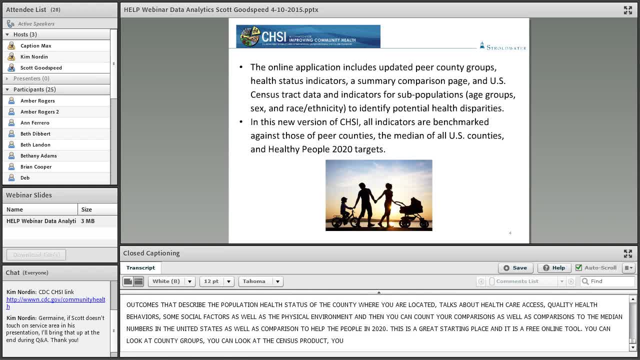 census tract. you can look at it for subpopulations by age group, say, sex, race, ethnicity. the other thing that in this version, all the indicators, as I mentioned, a benchmark against peer counties, the median of all US counties, and healthy people 2020 target, so it's a it's a very good place to to begin. 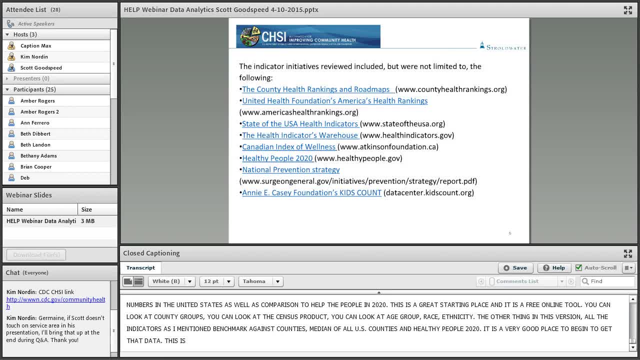 looking at data. this is the. this is the website that you can, you can go to and I just want to share. these are the, a whole list of other websites, as well as indicator initiatives that they reviewed. if you have time, I would suggest that you at least, at a minimum, visit the county health rankings and 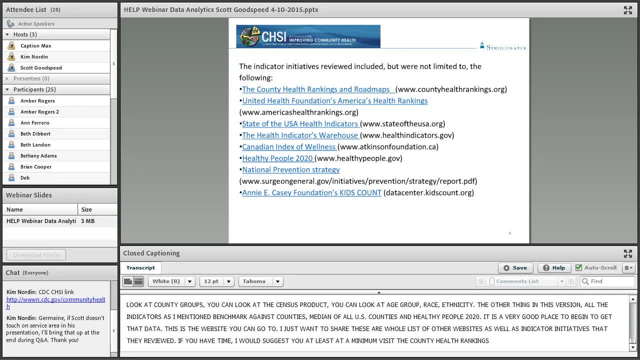 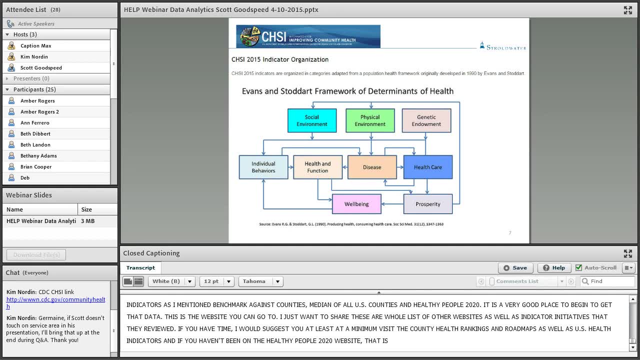 roadmaps, as well as the US health indicators, and if you haven't been on the healthy people 2020 website, that is another very, very good source you. so this, the framework that the CDC used, is it's: it's a little bit old, it's 1990. 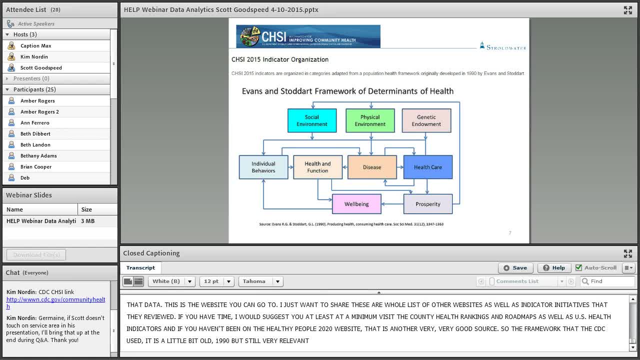 but it's still very relevant today and it's called the Evans and Stoddard framework for the four determinants of health and if you look down at the bottom pink purple box where it says well-being, basically the model that that the CDC is using has a hypothesis- hypothesis that there's certain things. 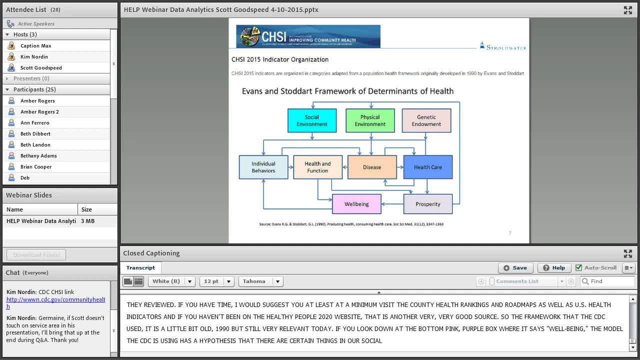 in, in in our social environment that may lead to individual behaviors- behaviors. there are certain things, if not physical environment, that may either promote or enhance disease. when we talked about blue zones on Wednesday, we learned that the research that came out of the National Geographic work that dan 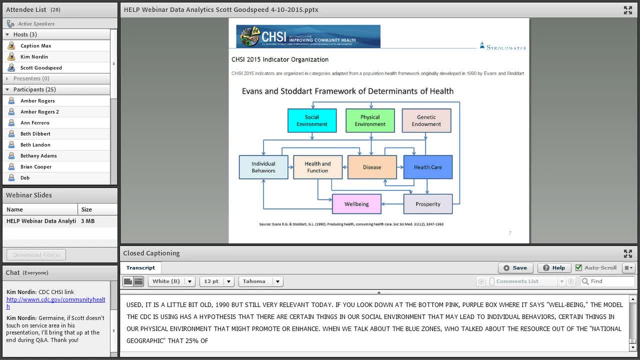 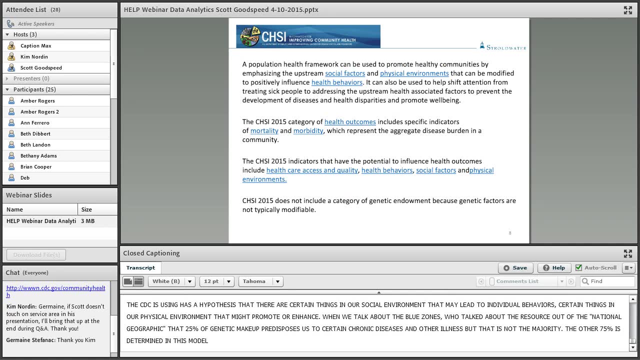 Buechner did that about 25% of genetic makeup predisposes us to certain chronic diseases and other illness. but that's not the majority. The other 75% is determined in this model here. So the framework can be used to promote healthy communities. They look at social. 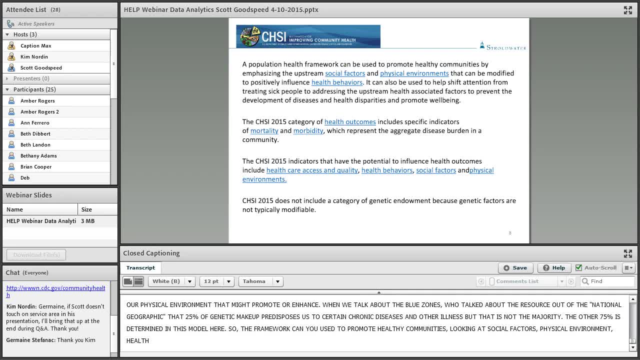 factors, physical environments, health behaviors, health outcomes, morbidity, mortality- And when you go to the website, you can see all of these indicators and you have indicator definitions. It's probably obvious, but this website does not have a category of genetic endowment because 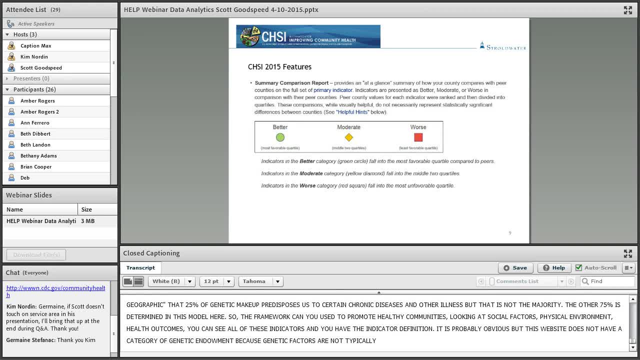 genetic factors are not typically modifiable. So when you go into the website and you type in your state and the county you're located, you're going to see a table like this and it's basically a summary comparison report and it gives you an at-a-glance. 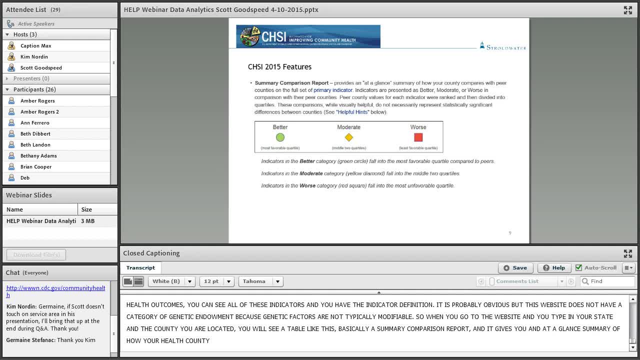 summary of how your county compares with peer counties for a full set of indicators. Now let me just tell you what the primary indicators are and I suggest when you go to the site you actually can click on primary indicator and you can see what the indicators are. So the 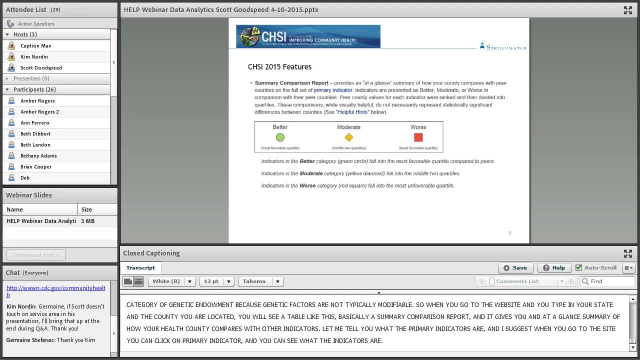 indicators are grouped in a bunch of different ways and you can see what the indicators are And I'll show you what it is. There are words and letters for different categories. For example, there are indicators related to mortality. So if you want to know mortality in your county by age, 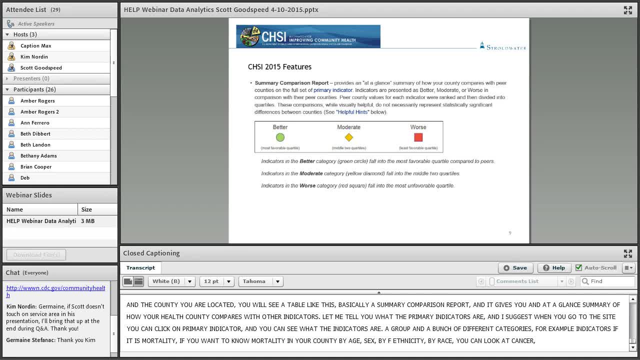 sex, by ethnicity, by race. you can look at cancer, diabetes, stroke, motor vehicles. If you want to better understand morbidity in your county, you can look at things like obesity and diabetes. If you want to understand healthcare access and quality, you can look at primary care provider. 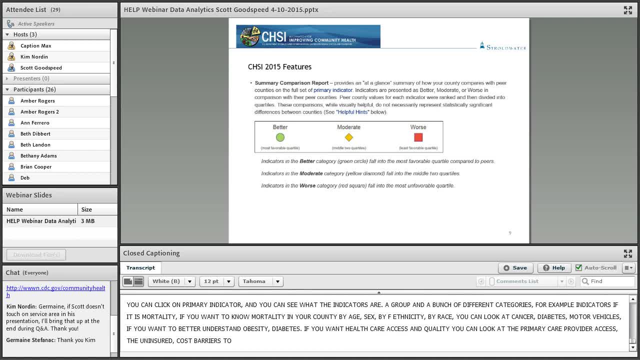 access. you can look at definition, you can look at acronyms, you can look at nameàs and you r kt ley E file of various information to ensure that your county sounds as concerned as Anaheim. look at the uninsured. you can look at cost barriers to care if you want to. 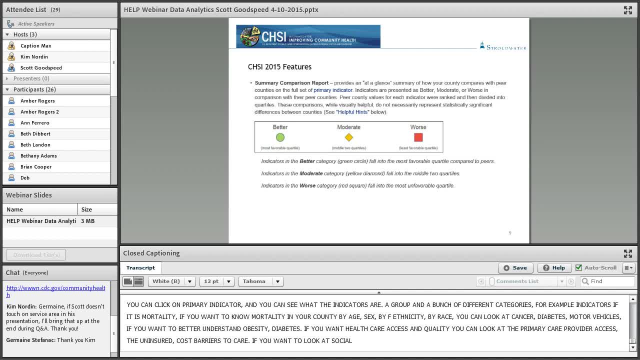 look at social factors. you can look at things like poverty, violence, children with single parents. if you want to look at healthy behaviors as a primary indicator, you can. you can click on that. and you can look at smoking, things like teen birth, physical inactivity. so so there's a lot of information that is. 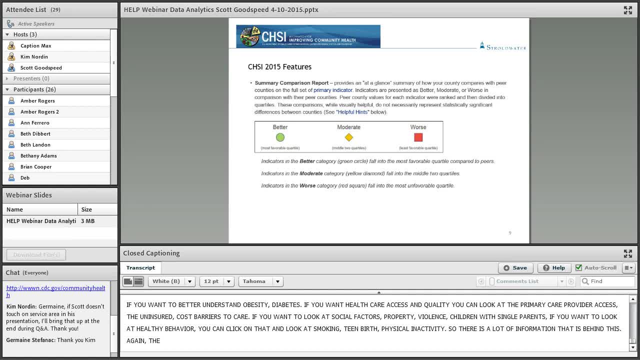 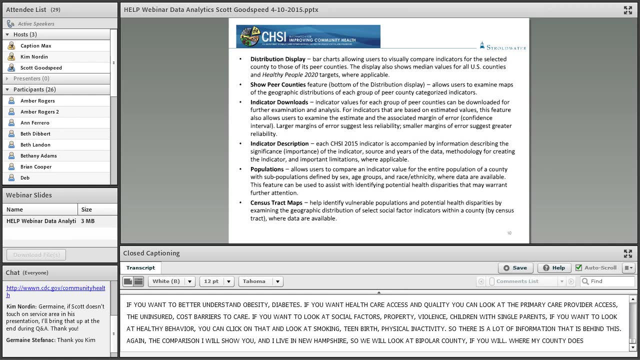 behind this. again the comparison that I'll show you. and I live in Rockingham County in New Hampshire, so we're going to look at my home county, if you will, and again, this is publicly available data, and we'll see where either my county does better than the peer group, better than the US median, or where it. 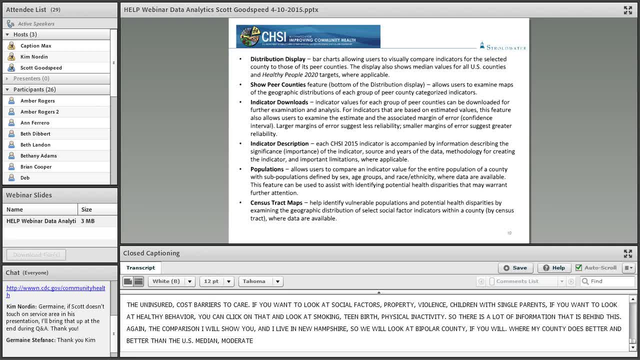 does moderate or worse. this is just some additional information that you can find on the site. there's a lot of information that you can find on the site. there's a lot of detailed information here. I'm not going to go through it, but I would just mention that there's an indicator description. so if you're presenting this, 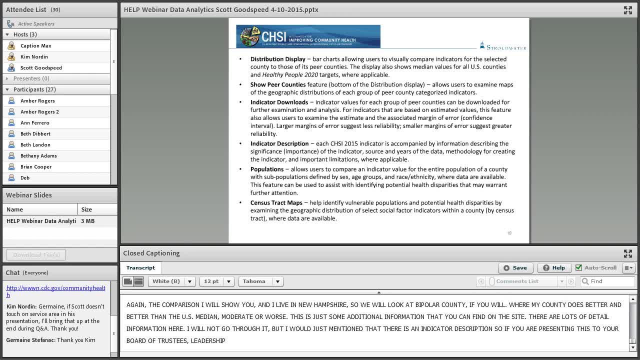 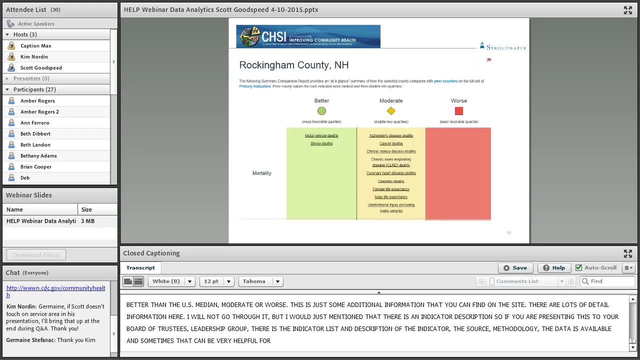 to your board of trustees, the medical staff leadership group. there is a, the indicator, listing a description of the indicator, the source, the methodology, the year that the data is. a is available and sometimes that can be very helpful for a internal or an external presentation. so this is my home County, Rockingham County in New. 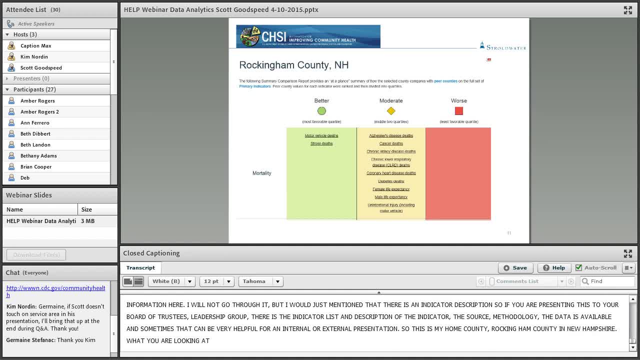 Hampshire, and what you're looking at is this comparison report at a glance. so all of these things that you see in the boxes- motor vehicle deaths, stroke decks, that- those are all what they call primary indicators and you can see for a motor vehicle deaths and stroke deaths, my county does better than its peer county. 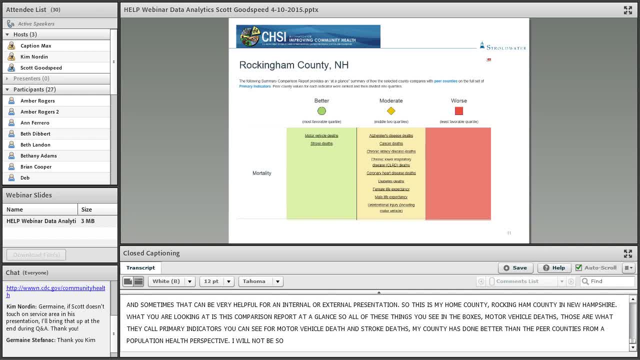 probably from a population health perspective, I'm not going to be so concerned about those kinds of causes of death when you go to the, to the middle box, where there's that moderate category I'm a little more interested in and things like chronic lower respiratory disease, coronary heart disease, diabetes. 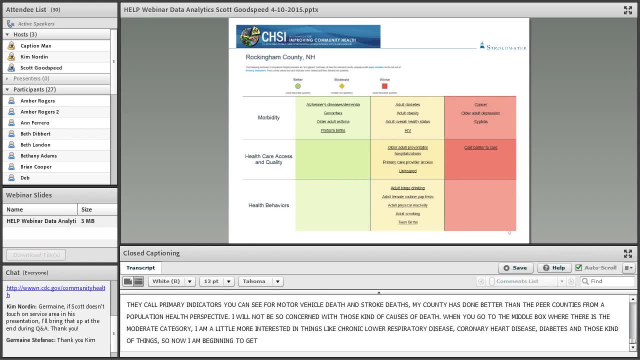 and those kinds of things. so now I'm beginning to get a sense of where I might look, at least with with this publicly available data. when we look at morbidity and I look at the moderate category now I'm very interested in diabetes and obesity and adult overall health status. if I go over 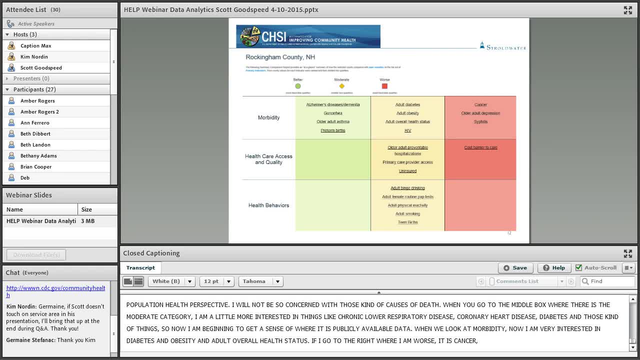 to the right. where I'm worse, you can see it's cancer and older adult depression. when you look at health care access and quality, there are some issues within my county related to primary care provider access in the uninsured. so what does that mean in terms of population health and visits to hospitals or visit to 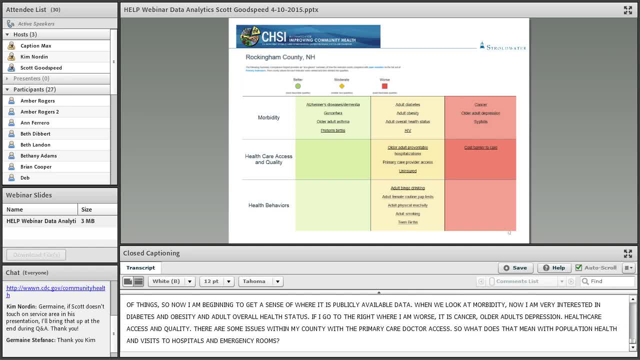 hospital emergency rooms. you can also see that when we look at health care access and quality, there are some cost barriers to care, so I'm very interested in that too. when we look at health behaviors and the moderate range- my county- there's an issue with adult binge drinking, adult physical inactivity, adult 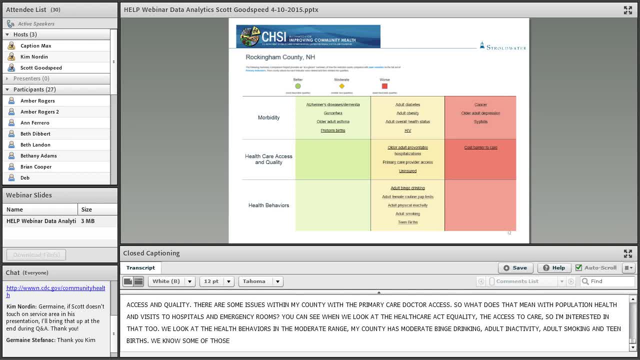 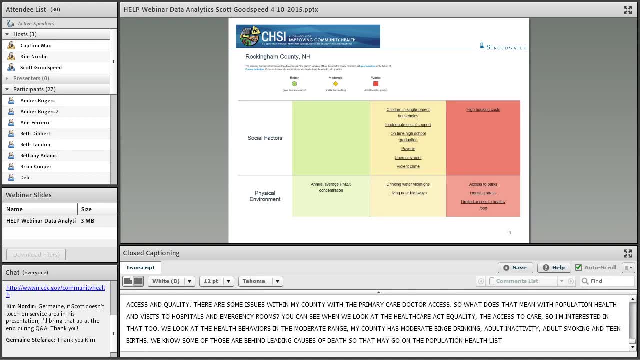 smoking and teen broken And we know some of those things are behind the leading causes of death. So that may go on my population health list agenda. And then, finally, when we look at some additional primary indicators, when we look at the social factors, we look at the number of children in single parent households. 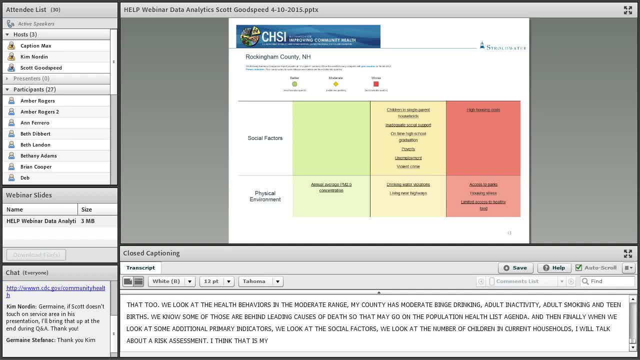 And I'm going to talk about a risk assessment- I think that's my last slide as it relates to kids and some of these other kinds of indicators. On time, high school graduation is an issue: poverty, violent crime, high housing costs- And then, if you look at physical environment, if you go to the far right-hand side, you 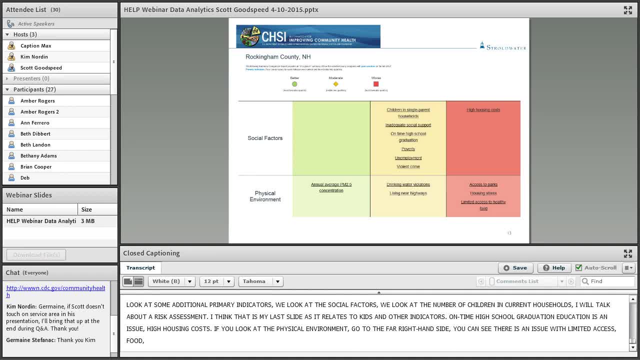 can see there's an issue as it relates to limited access to healthy food, And we saw that obesity in my county was a little bit of an issue. So we can begin to get a sense of kind of where we're going to begin to look at the 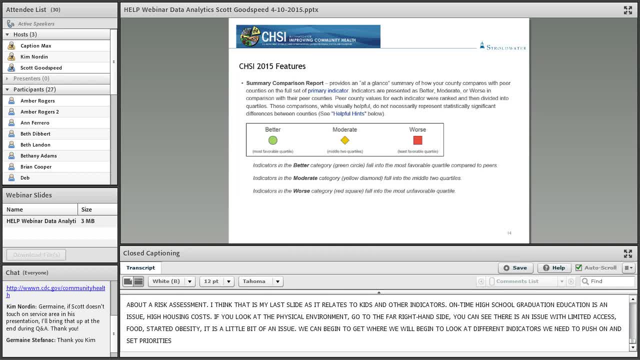 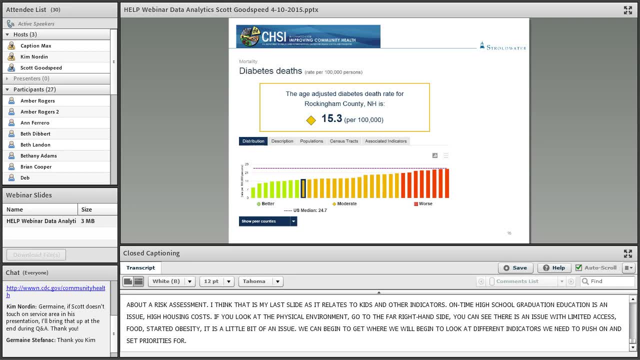 what kinds of indicators we need to push on and set priorities, for These are actually duplicate slides. The other thing: if I'm interested in diabetes deaths in Rockingham County I can get the rate per 100,000, and you can see that my county is below the US median. 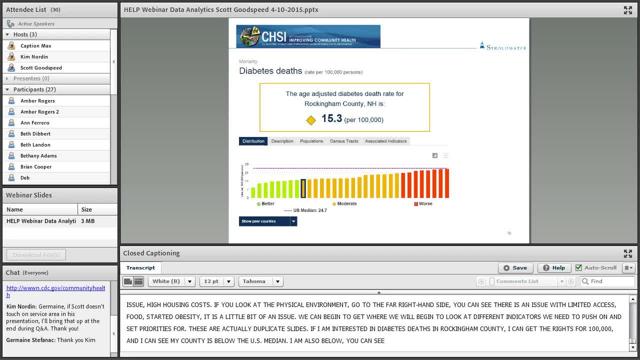 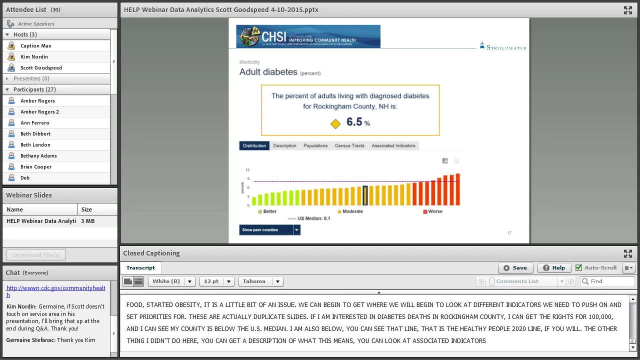 I'm also below. You can see that That dotted line that's the Healthy People 2020 line, if you will- The other thing that I didn't do here you can get a description of what this means. You can look at census tracts and you can look at associated indicators here. 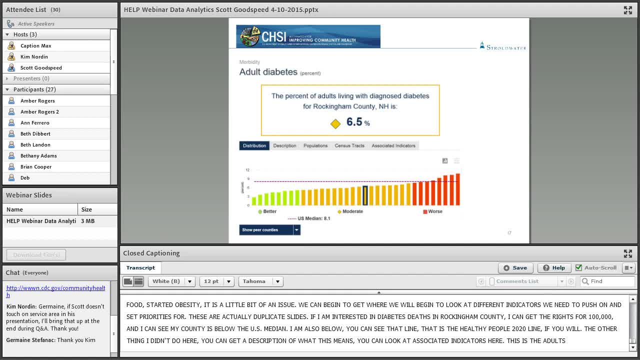 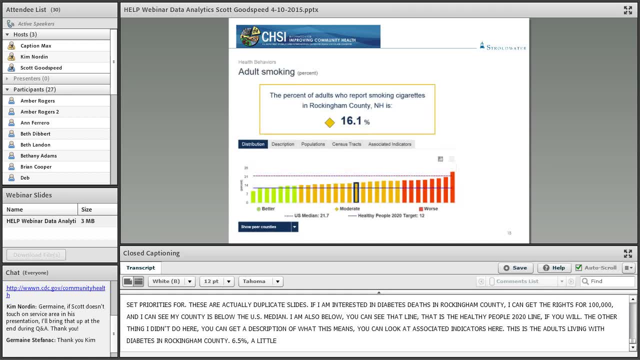 This is the percent of adults living with diagnosed diabetes in Rockingham County at 6.5%. You can see It's a little bit less than the US median. When we look at the percent of adults who report smoking cigarettes in my county it's 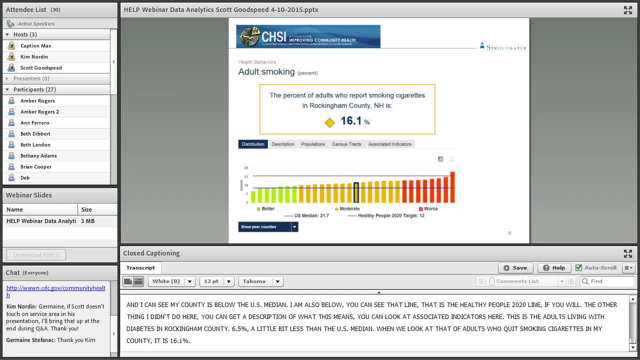 16.1%. So, even though it's a little bit less than the US median, it's over, It's greater than the Healthy People 2020 target And again, I mentioned the Healthy People 2020 website. If you want to set targets in your community that are consistent with your target, you. 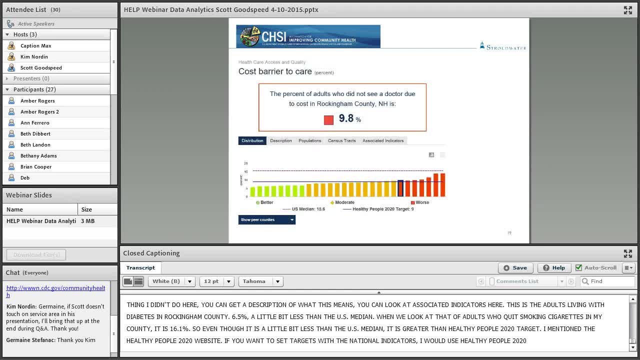 may want to set some of the indicators. I would think within 70% of the population who are these places in Rockingham County, a bunch of people in my county who are people health Easel that are stream, obviously Having their data screaming on all of the кар Province down here you can tell they're. 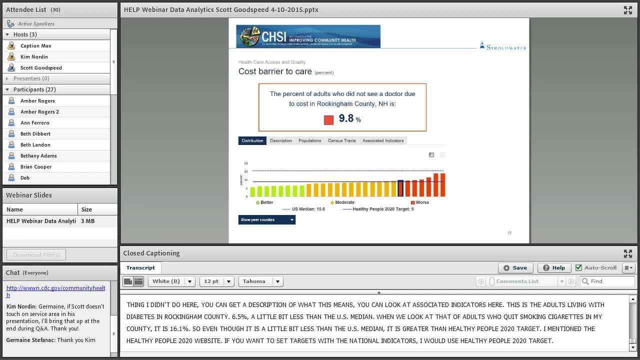 really important. And then, ultimately, when you go back, if anybody who is going to make their time to think in such a more healthy and efficient way is, with some of the national indicators, I would use the Healthy People 2020 targets. This is the percent of adults who didn't see a doctor due to a cost in Rockingham County. You can see it's 9.8%. It's less than the US median, but it's hovering right around the 2020 Healthy People target. 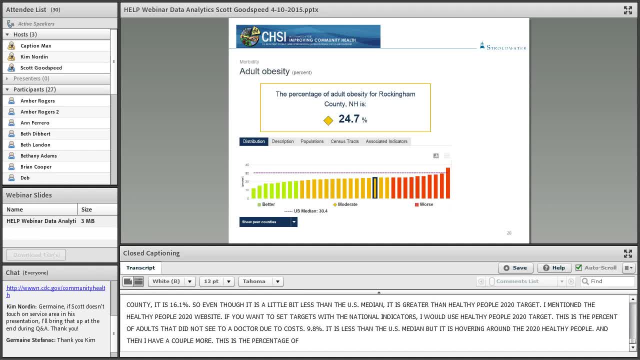 And then I think I've got a couple more. This is the percentage of adult obesity. the percentage of adult obesity for Rockingham County: It's 24.7%. You can see it's less than the US median, but I'm in this category of this kind of moderate category. 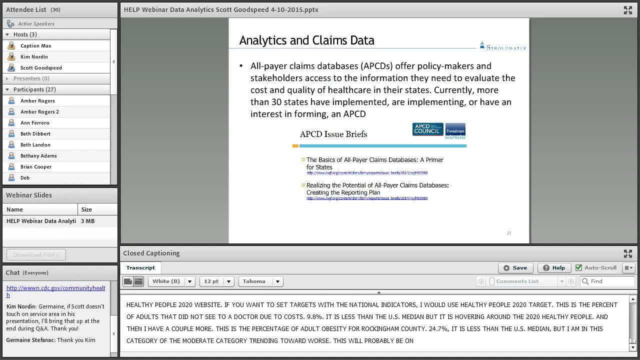 trending to worse. So this is probably gonna be on my list in terms of one of the population health initiatives. So I would encourage you- and you can spend hours on that website. I would encourage you for your state and your county to look at your indicators. 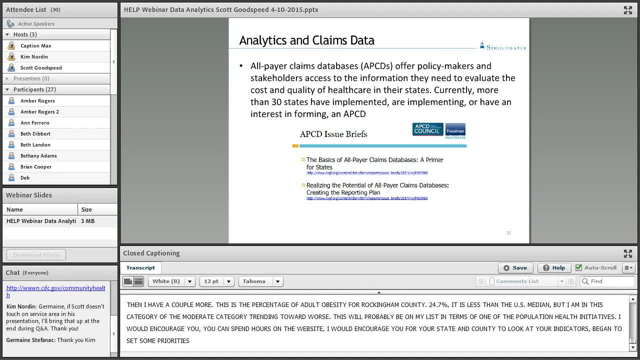 begin to set some priorities using that website, And now we're gonna go the next level down and dig a little bit deeper. So we talked about publicly available data. Now I'm talking about data that's privately available. However, as we go through this part of the presentation, 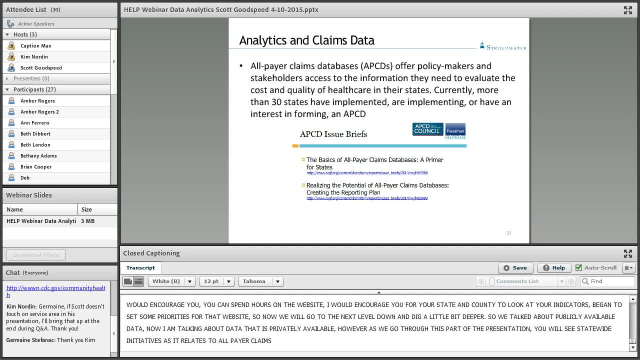 you're gonna see some statewide initiatives as it relates to all payer claims databases. So now we're talking about analytics and claims data And I'll tell you specifically what that is. So there are all payer claims databases that offer all of us a chance to look at information. 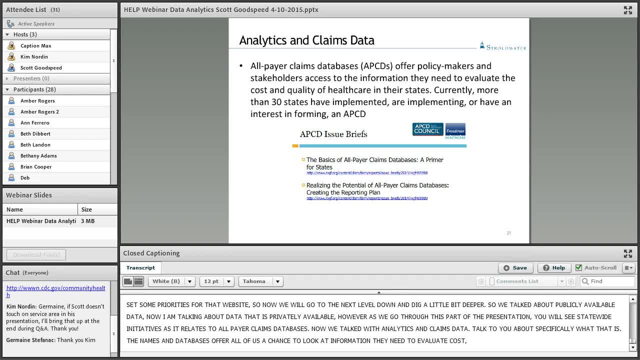 they need to evaluate cost, quality, incidence, prevalence of disease And right now there are more than 30 states that actually have implemented all payer claims databases And I'll show you a map and you can see if your state is one of those that is participating. 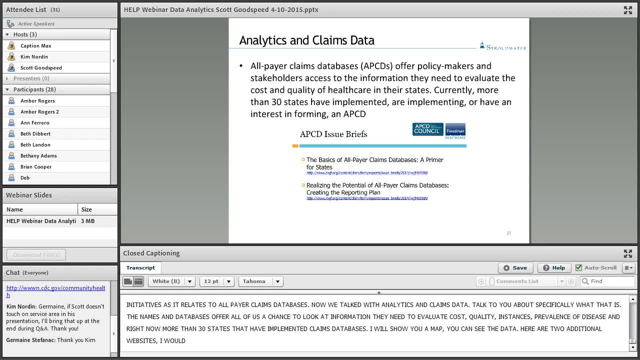 Here are two additional websites. I would check those in the next week or two. And the second website is a very good source because it talks about how you can realize the potential of claims databases and how you can come up with a plan to report those data publicly as well as publicly. 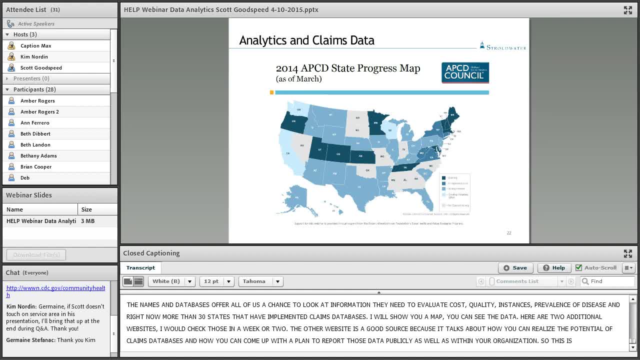 As well as within your organization. So this is a 2014 map, as of March 2014,, with the all payer claims database, And you can see where you see the gray, those are states that have no current activity today. The dark blue: that's where there are. 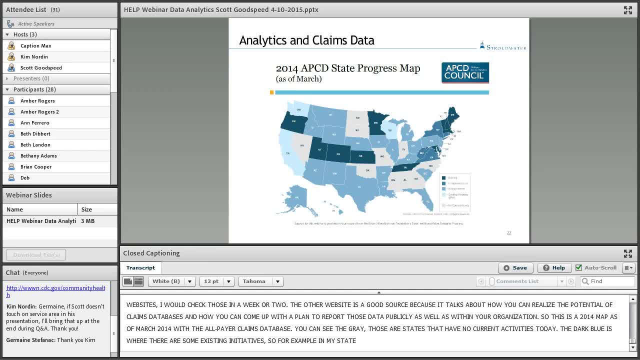 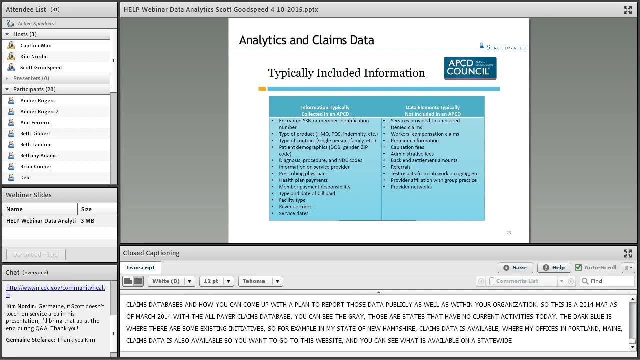 some existing initiatives. So, for example, in my state of New Hampshire claims data is available. Where my office is in Portland, Maine, claims data is also available. So you want to go to this website and you can see what's available on a statewide basis. 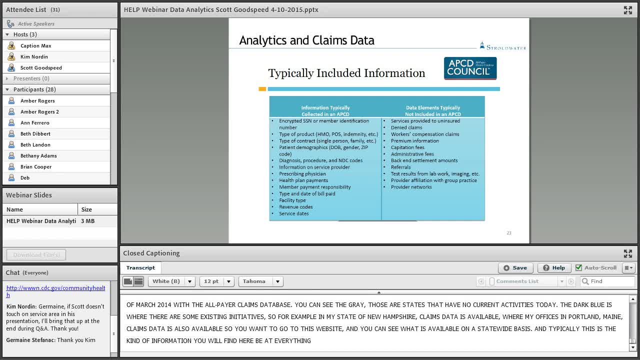 And typically this is the kind of information you're gonna find here, And everything is encrypted. So it's encrypted. social security numbers, patient identification, of course, is encrypted. You can look at types of products. You can look at patient demographics. 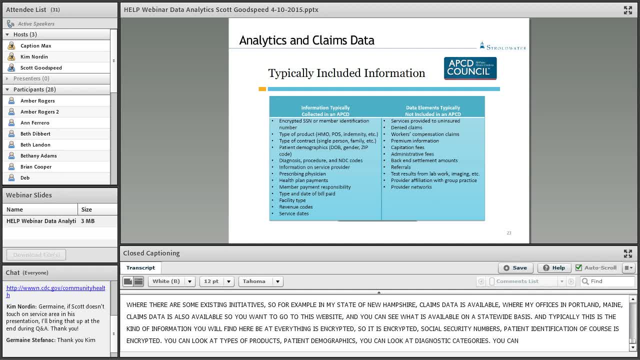 You can look at diagnostic categories, You can look at procedures, You can look at health plan payments. You can look at facility types. You can look at revenue codes. On the right hand side are the kinds of data elements that you're typically not gonna find in this database. 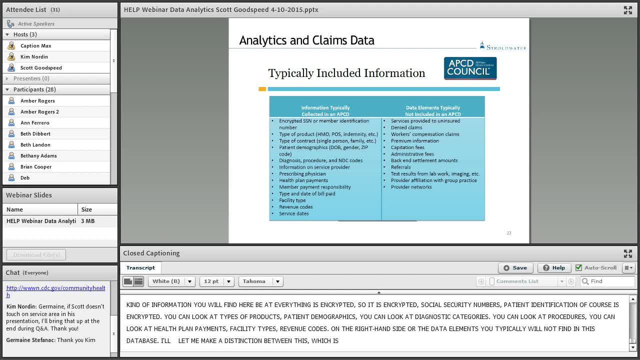 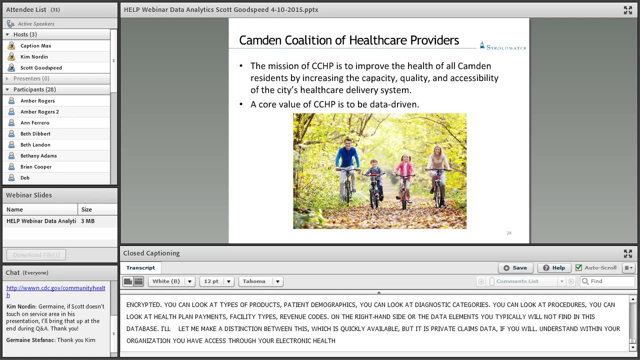 Now, let me make a distinction between this, which is this, Which is publicly available, but it's private claims data, if you will Understand that, within your organization, you have access to, through your electronic health record, your own claims data. 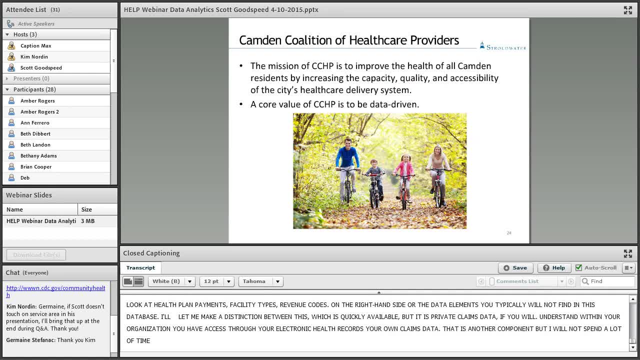 So that's another component, but I'm not gonna spend a lot of time talking about that, So here's one. this is the state of New Jersey and this is how they used it, And the Camden Coalition of Healthcare Providers, and you'll have their website. 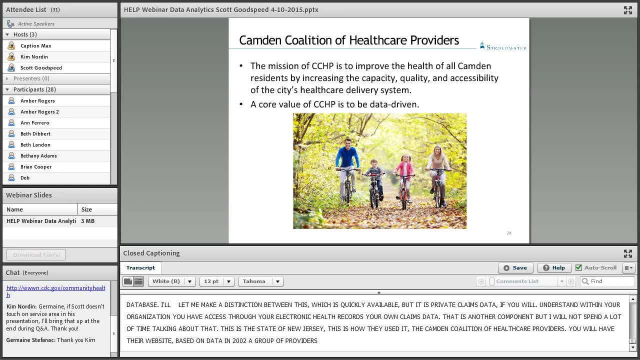 they started in 2002.. A group of providers came together and they decided that what they wanted to do was to improve the health of Camden residents by increasing capacity, quality, accessibility of the city's healthcare delivery system. And you're gonna see some screenshots. 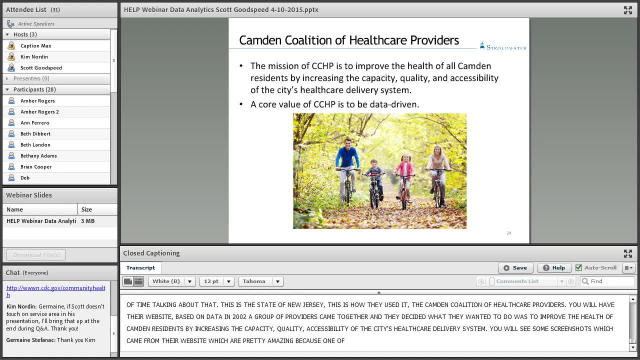 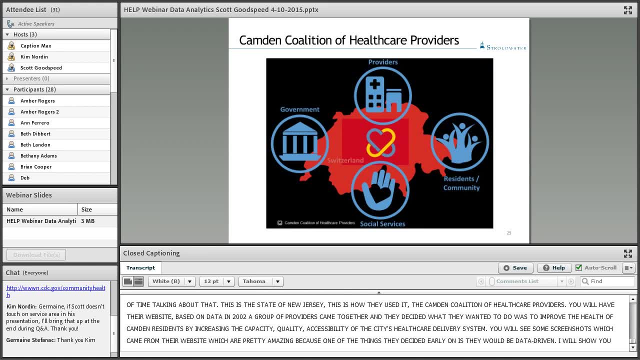 which came from their website that are pretty amazing, because one of the things that they decided early on is that they would be data driven, And I'll show you what that specifically means. So this coalition of providers, so it was hospitals, it was other healthcare organizations- 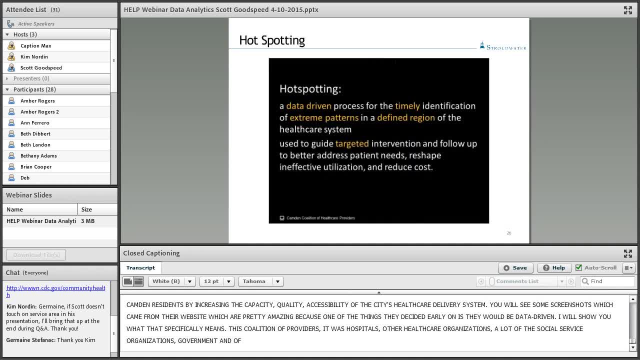 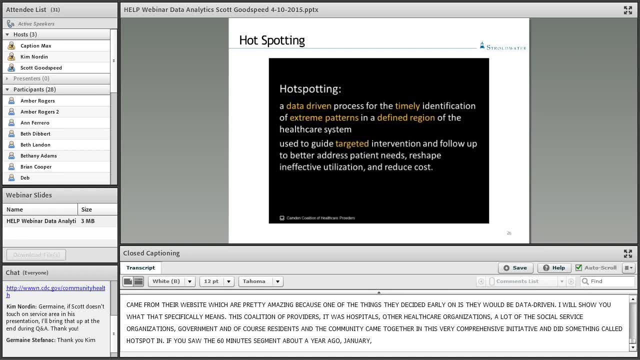 about a year ago- January, February 2014.. They actually had a segment on hotspotting and the use of big analytics, if you will. So hotspotting is a data driven process for the identification of extreme patterns in a defined geographic region. 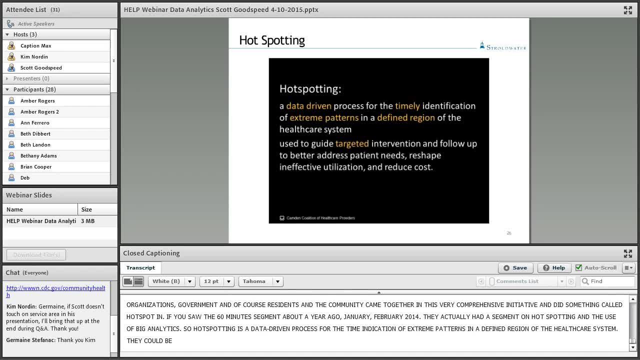 It could be a county, it could be a city, it could be a building, And I'm actually gonna show you some of the buildings in Camden, New Jersey, that represent populations with the highest use rates, the highest falls. So we can use this hotspotting technique. 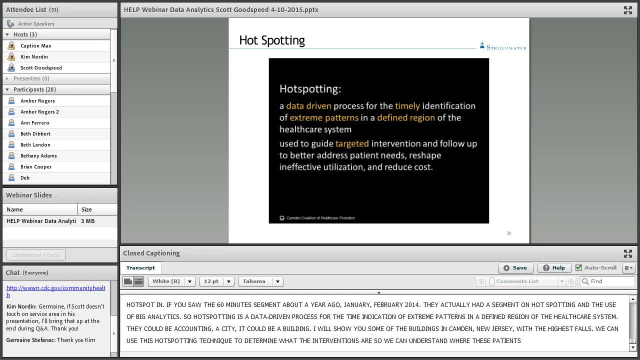 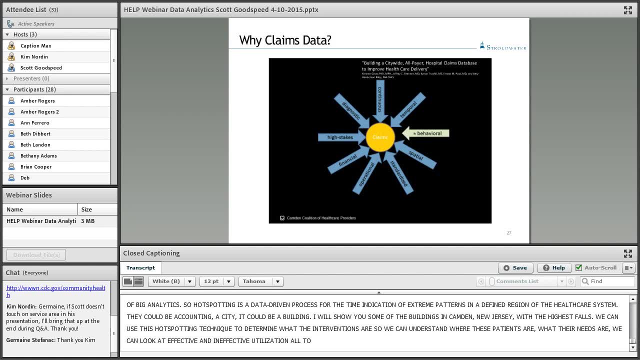 to determine what the interventions are, So we can understand actually where these patients are, what their needs are, We can look at effective and ineffective utilization- all to reduce costs and to improve quality. So the group came together and built a claims database. 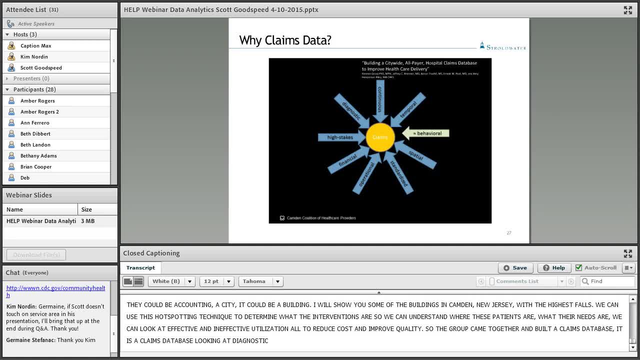 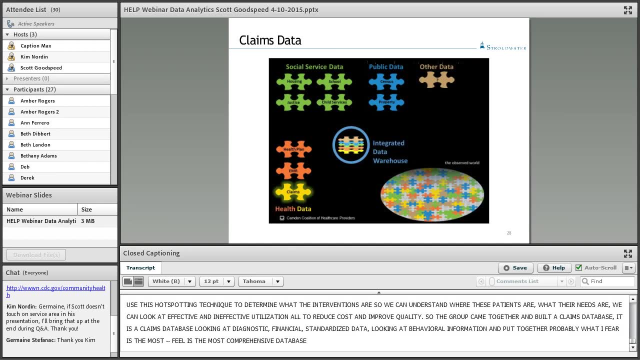 So it's a claims database looked at diagnostic, financial, operational, standardized the data. They looked at behavioral information and put together probably what I feel is one of the most comprehensive claims database that's actionable in the United States. So they had all of the social service organizations. 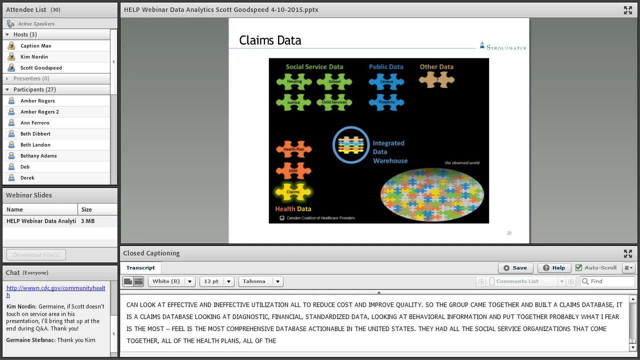 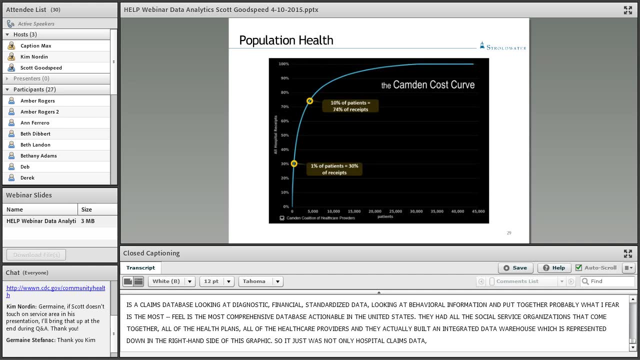 come together, all of the health plans, all of the healthcare providers, and they actually built a integrated data warehouse, which is represented down in the right-hand side of this graphic. So it just was not only hospital claims data, it was comprehensive claims data. 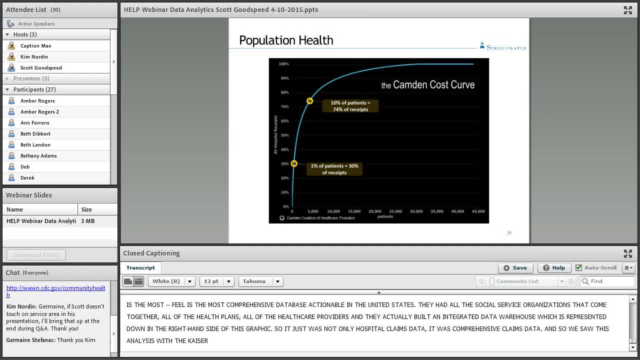 And so we saw this analysis with the Kaiser Family Foundation and this is what showed up in the Camden, New Jersey at the healthcare coalition. And this is their cost curve. So when they looked at all of the claims there, they found out and determined that 1% of their patients okay, equals about 30% of the receipts or of the hospital spending. Again, 1% of the patients represents 30% of the spending, And we talked about that when we looked at some of the national data last time. What's also very interesting is is 10% of the patients. 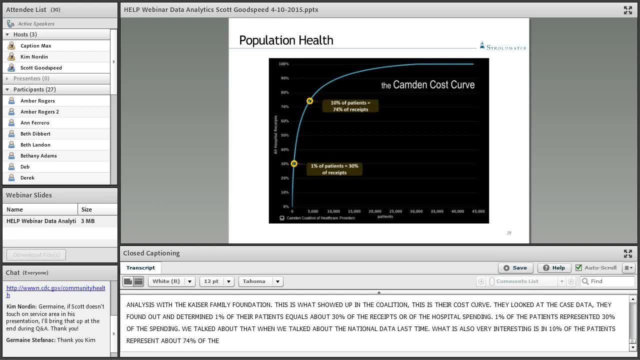 okay, of the hospital spending is 10% of the patients. 10% of the patients represent about 74% of the receipts. So if you actually look at the numbers here in Camden, that represents about- I think it was about- 5,100 patients. 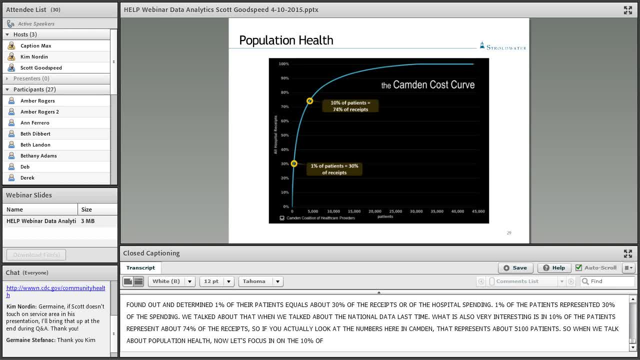 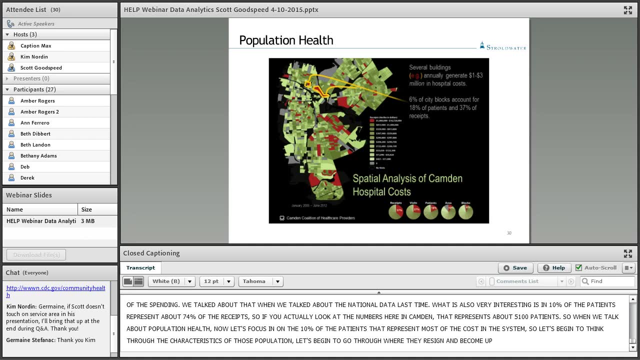 So when we talk about population health now, let's focus in on those 10% of the patients that represent most of the cost in the system, And so let's begin to think through the characteristics of those population, Let's begin to think through where they reside. 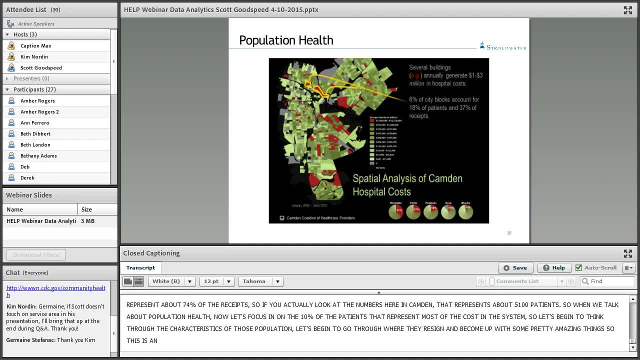 And you actually begin to come up with some pretty amazing things. So this is an example of hotspotting, And this is in Camden, New Jersey, where it's a little bit difficult to read, but you can see where these yellow lines go represent several buildings in Camden, New Jersey. And they annually generate one to $3 million in hospital costs. just those buildings And so 6% of the patients. that represent 7% of the city blocks, account for 18% of the patients and 37% of the receipts. So now with the hotspotting and looking at the map, 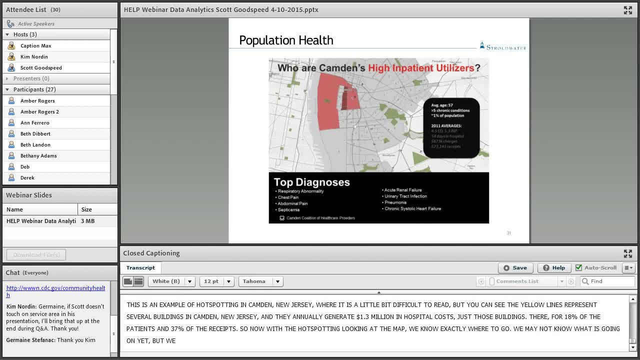 we know exactly where to go. We may not know what's going on yet, but we will Now when we want to understand Camden's high utilizers. the average age is 57. They typically have greater than five chronic conditions, and that represents 1% of the population. 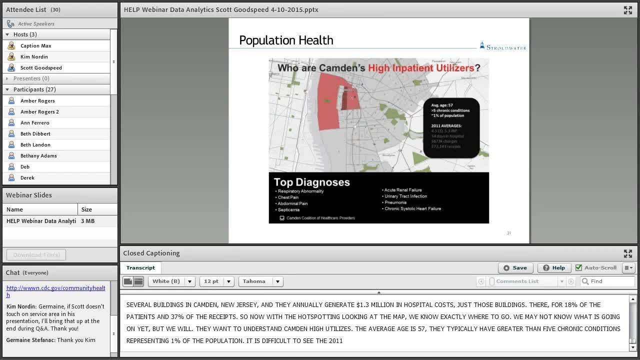 It's difficult to see the 2011 averages, but they typically spend 54 days in a hospital, $673,000 in discharges, And typically spend four and a half ED visits And, as I mentioned, 54 days in the hospital. 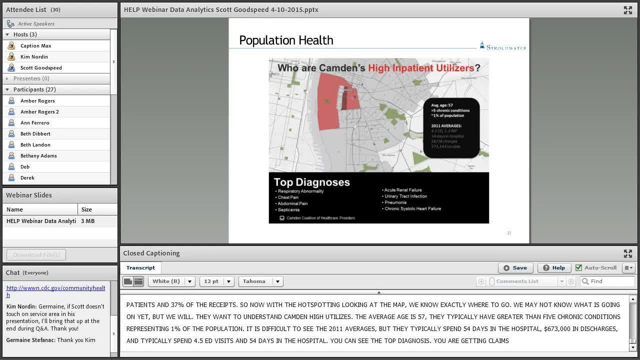 and you can see their top diagnosis. And again you're getting that from the claims data. So these patients are on their first day of hospitalization. And again you're getting that from the claims data. So these patients- and once again we're talking about high治gant patients- 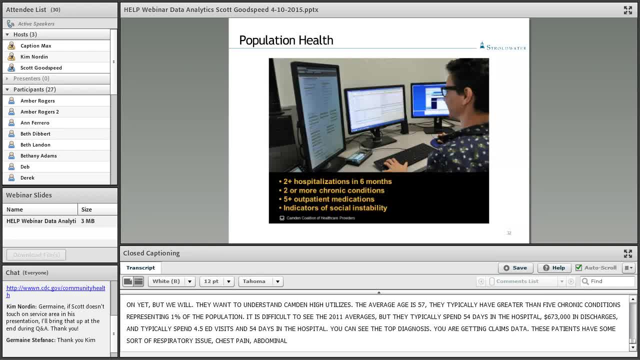 Patients either have some type of respiratory issue, chest pain, abdominal pain, and you can see the list. So that's where we're going to begin to focus And this is a little more specificity in terms of this patient population. They have two plus hospitalizations in six months, two or more chronic conditions. five: 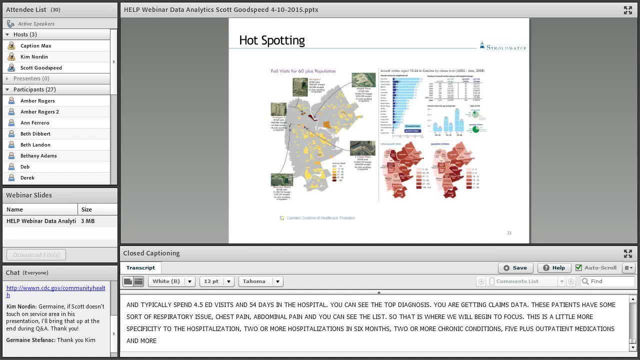 outpatient medications and there are some different indicators that they look at as it relates to social instability. This is very difficult to see and I apologize, but this is hotspotting and what we're doing is actually looking at fall visits for the 60-plus population and the way that 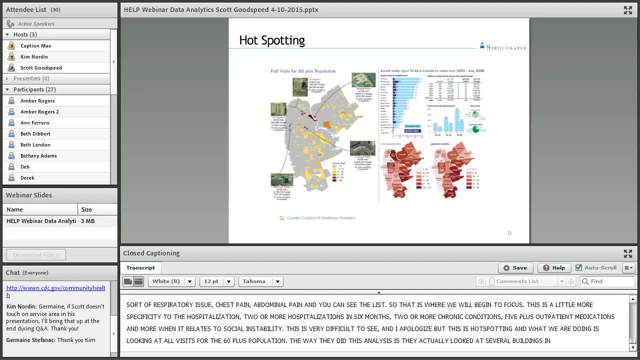 they did this analysis is they actually looked at several buildings in Camden and, while this is difficult to read, for each building it's got the number of falls, the total number of receipts or the total spending related to those. So one of the initiatives that you find in Camden is a fall initiative. 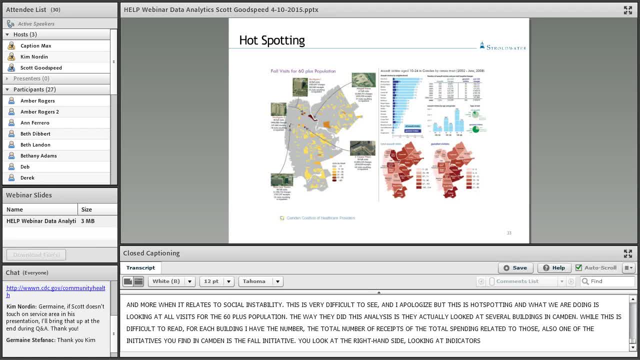 If you look at the right-hand side, they're looking at indicators such as assault victims, total assault visits, gunshot victims and while the Camden graphic is a little small, you can see where they hotspotted that and they know they have some specific issues. 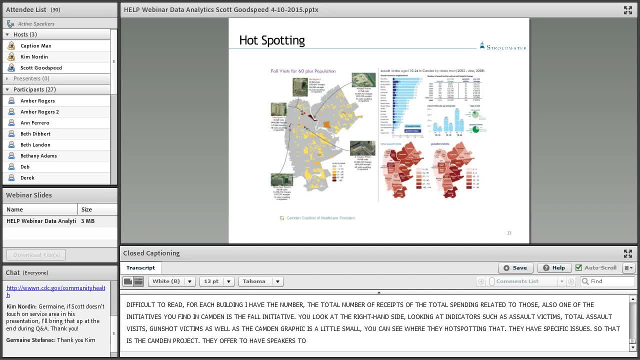 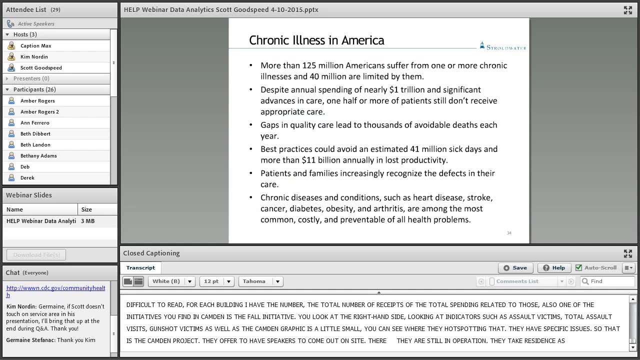 So that's the Camden project. They offer to have speakers to come out on site. They're still in operation. They have, you know, they take residents and interns, and so this website again is another very, very, very good source as it relates to population health. 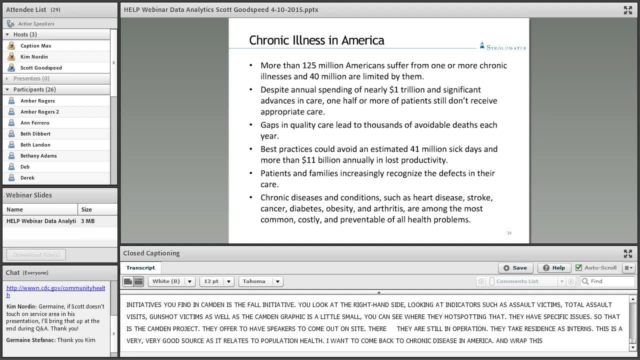 So I want to come back to chronic disease in America and I'm going to wrap this up in about 10 to 12 minutes, Thank you. So we talked about on Wednesday how more than 125 million Americans suffer from one or more chronic diseases and 40 million are limited by them. 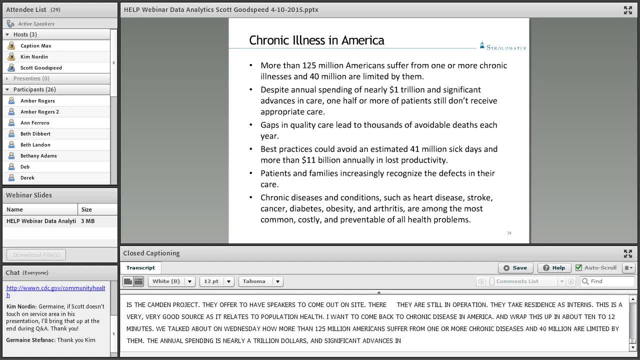 The annual spending is nearly a trillion dollars and there are significant advances in care, but we also know one-half or more of the patients still don't receive appropriate care, So there are gaps in the quality that lead to thousands of avoidable deaths each year. 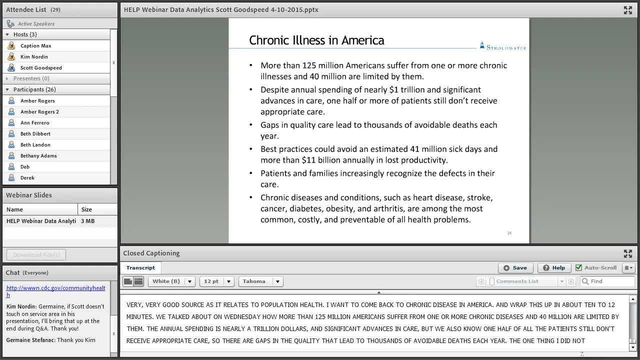 Thank you. The one thing that I didn't spend any time on that we should pay attention to is the whole issue of readmissions and the ambulatory sensitive conditions, particularly as it relates to those potential patients over 65, because those admissions for those ambulatory sensitive. 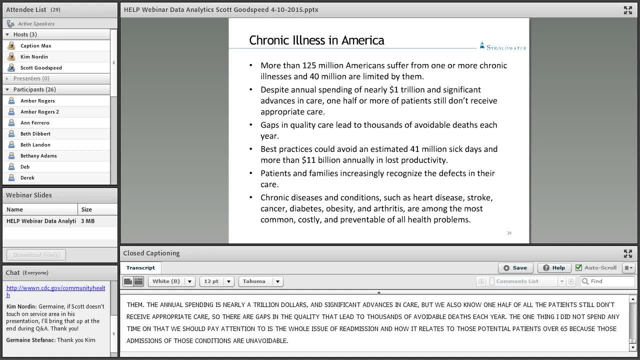 conditions are unavoidable And you have all of that data in each of your organizations, Thank you. So the other thing that we know that best practices could avoid about 41 million sick days and more than $11 billion annually in lost productivity. So patients and families increasingly recognize that there may be some gaps in their care. 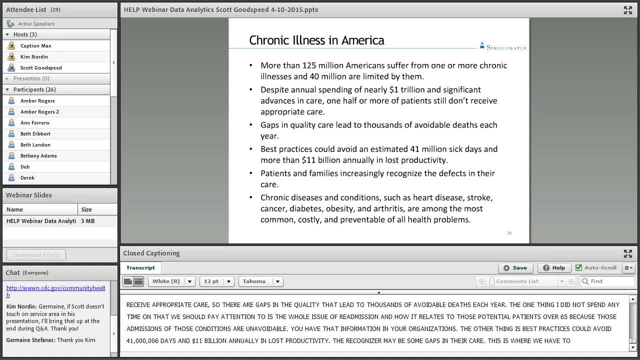 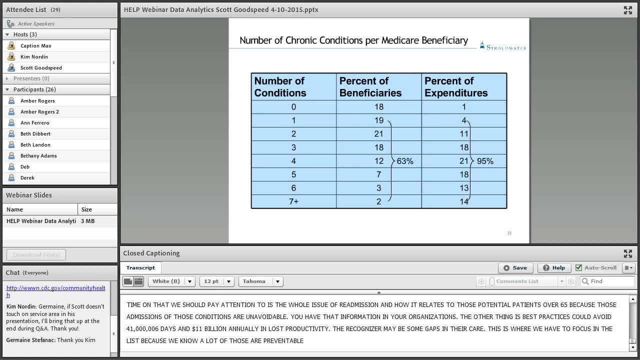 and we've talked about those chronic diseases and this is where I think we need to focus: heart disease, stroke, cancer, diabetes, obesity and down the list- because we know a lot of those are preventable issues. Thank you, If we think about Medicare beneficiaries- and again this is where we started the conversation- 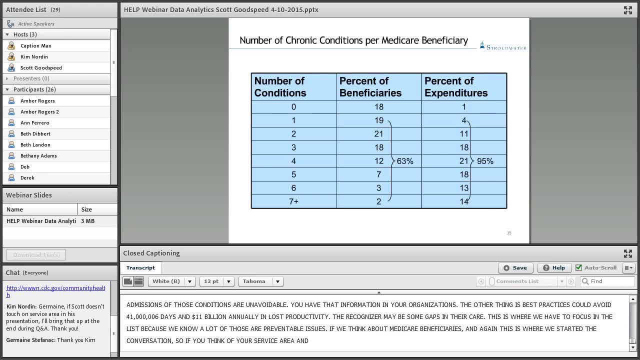 So if you think of your service area and all of the Medicare beneficiaries, whether they come to your organization or whether they go outside your service area to another organization, this chart shows the number of chronic conditions by percent of beneficiaries and the percent of expenditures. 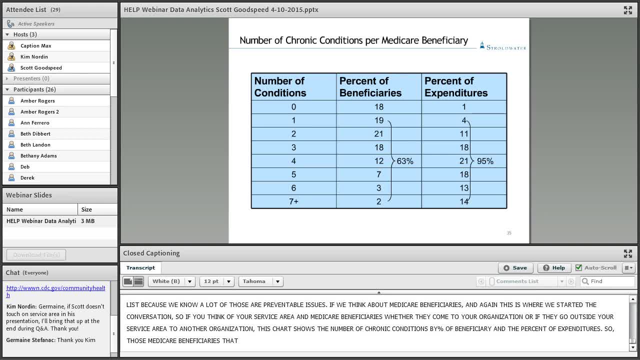 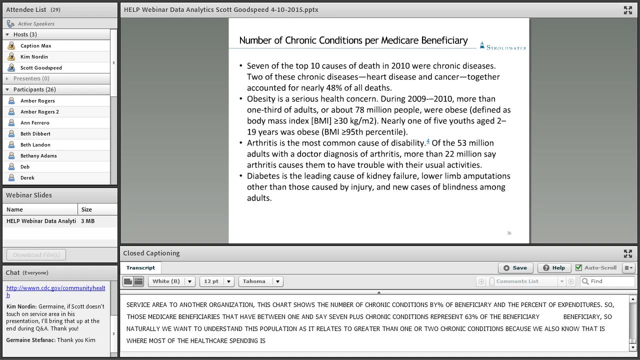 So those Medicare beneficiaries that have between one and, let's say, seven plus chronic conditions represent about 63% of the beneficiaries and about 95% of the cost. So naturally we want to understand this population, particularly as it relates to greater than one or two chronic conditions, because we also know that that's where most of the healthcare 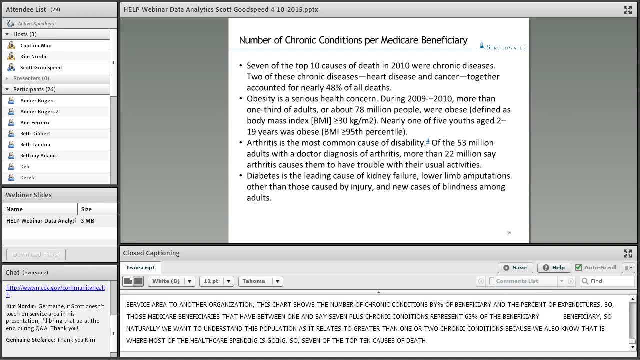 spending is So. seven of the top 10 causes of death in 2010 were chronic diseases. two of those chronic diseases- heart disease and cancer- accounted for nearly 48% of all the deaths. Obesity is a serious concern: more than a third of the adults of about 78 million people. 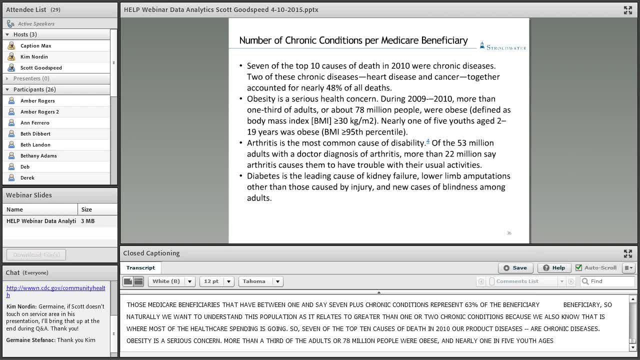 were obese and nearly one in five youths age two to 19 was obese. And again, you can get this all on the CDC, Thank you. So that's the CDC website for your county. Arthritis is the most common cause of disability. 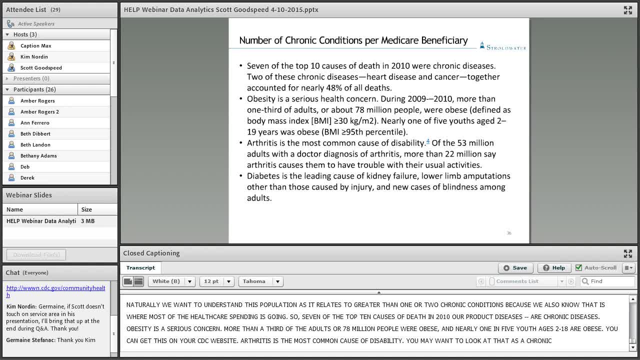 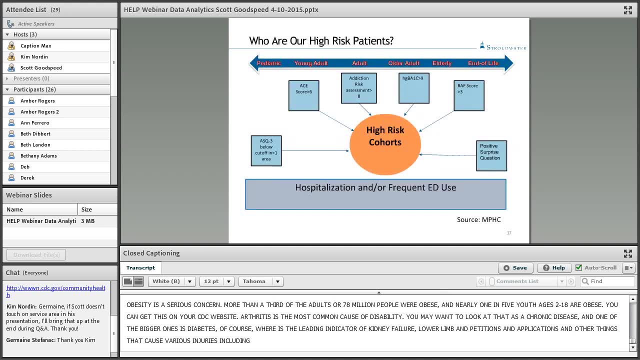 We may want to look at that as a chronic disease, And then one of the bigger ones is diabetes. Of course, we're the leading indicator of kidney failure. lower limb amputations and other things that cause various injury, including blindness, relates to diabetes. 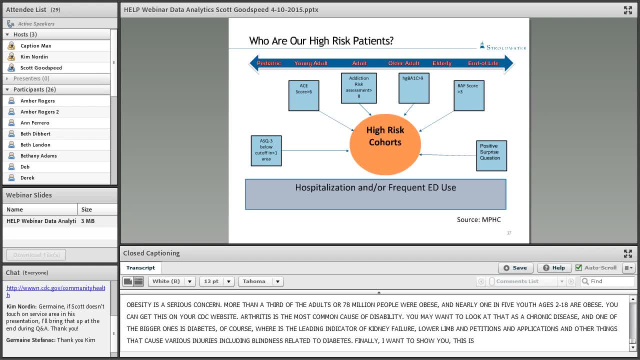 Finally, I want to show you this is MPHC, is Martin's Point Healthcare. We're doing some work with them today And this is one way of thinking through if you want an approach to understanding those high-risk cohorts. this is one approach with a number of indicators. 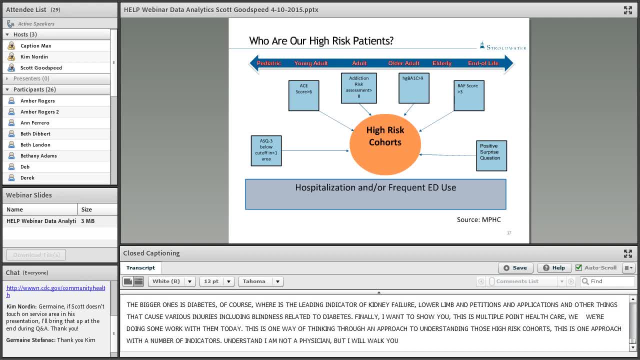 Understand, I'm not a clinician, I'm not a physician, but I'm going to walk you through this. So, first of all, we want to understand who are our high-risk patients: Those pediatric population, those young adults, adults, older adults, elderly. and then, as 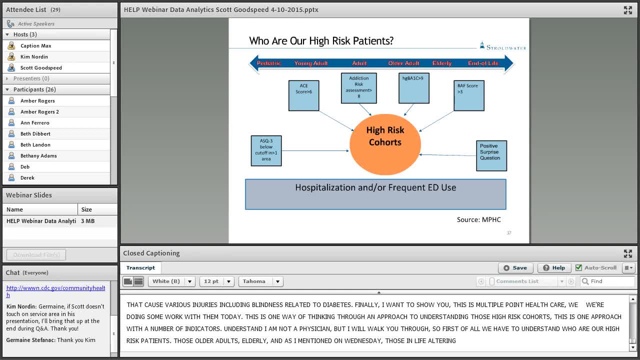 I mentioned on Monday, those in end-of-life situations. So here are some things to think about This ASQ-3 below cutoff in greater than one area. if you Google ASQ, you'll understand that that's the ASQ-3.. 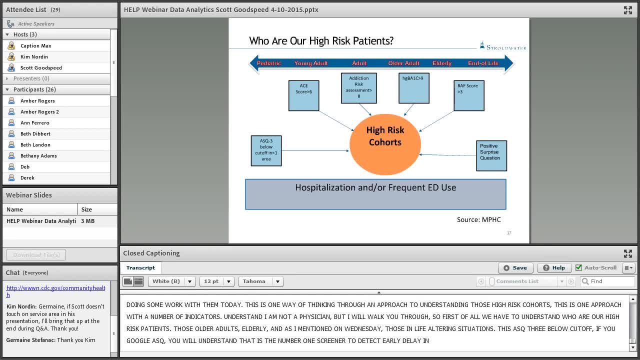 It's the number one developmental screener to detect early delay in children, And so they've got a criteria here that they want that number, the ASQ-3, below a cutoff score. but this could give you an indication of children that might be at risk. 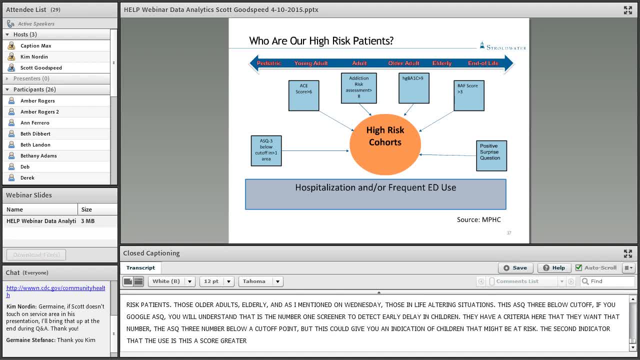 The second indicator that they use is this ACE score greater than six. Okay, So there are 10 types of childhood trauma, things like divorce, death, an alcoholic parent- And this score based on these indicators. they want to look at these kids who are at. 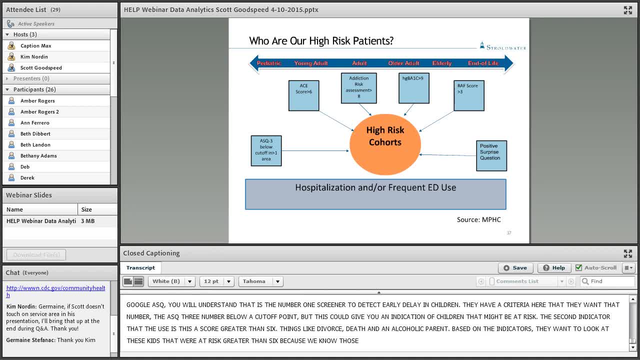 risk who have a score greater than six, because we know those kids may, or most likely will, fall into a high-risk cohort. This addiction risk assessment includes things like tobacco And alcohol And an assessment where they are a greater than a score greater than eight. 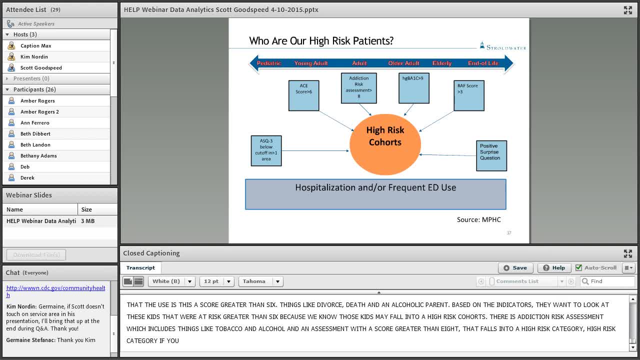 Again, that falls into a high-risk category, a high-risk population, if you will. The HDB1A1C is a diabetes predictor, And so they're saying, with a score greater than nine, those are the kinds of patients that we're very interested in following. 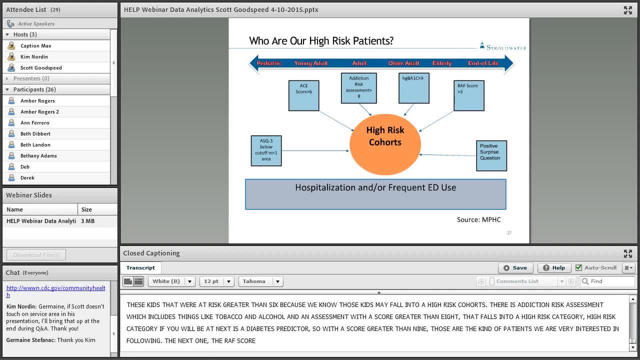 The next one is the HIV-A1C, The next one the RAF score greater than three. my understanding is that's a protein expression that correlates with breast cancer metastasis. So they're looking at a score greater than three and they're interested in that high cohort. 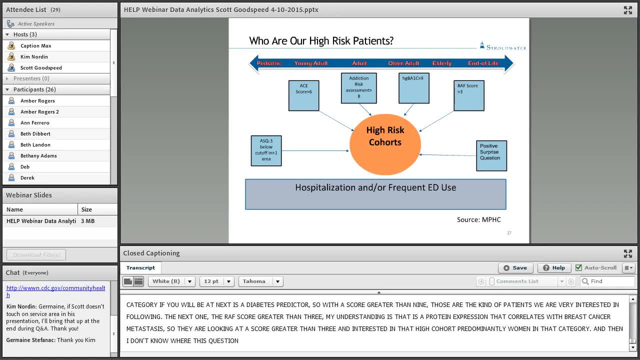 of predominantly women in that category. And then I don't know where this question came from, but it was what they call the positive surprise question. So if you go back in and ask your providers, so your physicians, nurse assistants, your PAs, 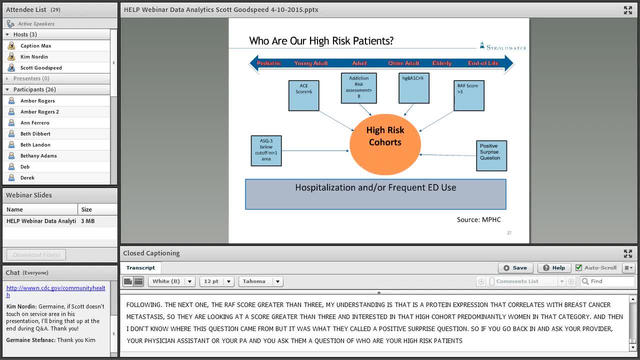 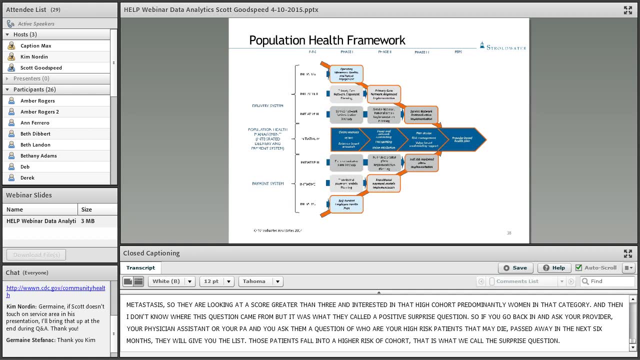 and you ask them the question of who are your high risk patients that may die, pass away in the next six months, they're gonna give you the list. Those patients fall into a high risk cohort too, and that's what we call the surprise question. 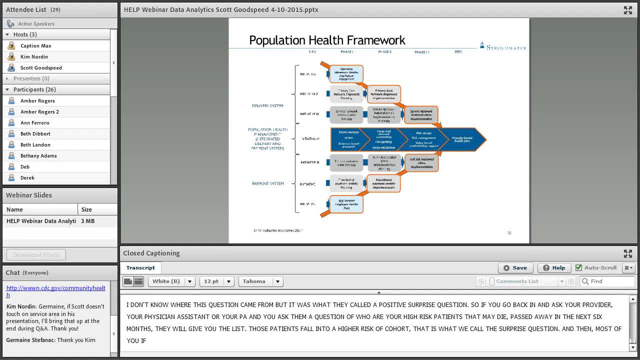 And then most of you, if you want a prior Webex. you've seen this population health framework. You may have seen Eric Schell or others from Stroudwater spend about an hour and a half or two hours to walk through this. 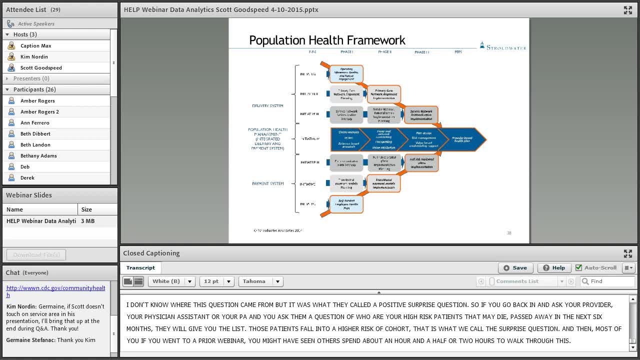 I'm not going to do that, but if you want a copy of this presentation in a PDF format, I'm more than happy to send it. But one very good place to start with. a board of trustees, a medical staff leadership group, an executive. 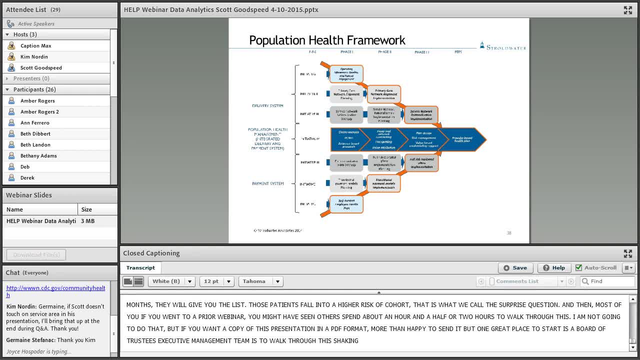 an executive management team is to walk through what we call this shaky bridge framework, if you will, Because one of the things that we do here is we specifically walk through the eight or nine initiatives that will eventually help you move from fee-for-service medicine. 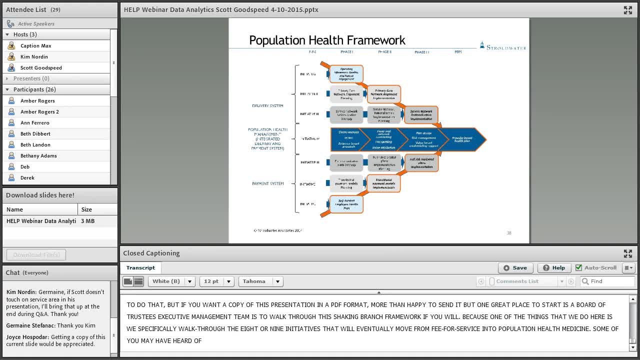 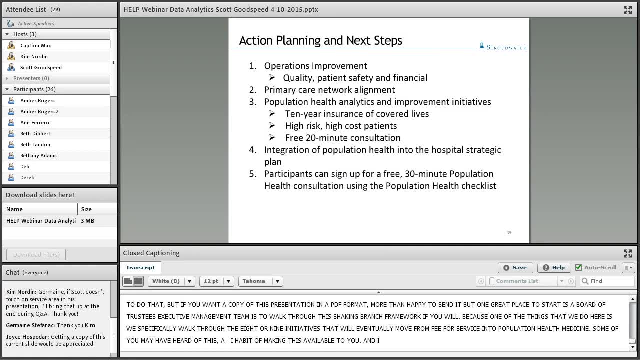 into a population health framework, And some of you may have heard this and again, we're more than happy to make this available to you. And then I think I've got one final slide in terms of action planning or next steps, Typically consistent with: 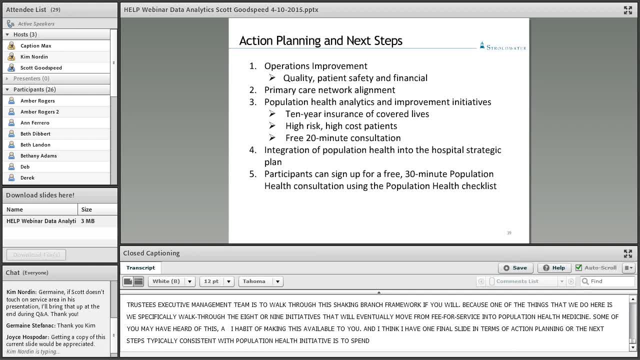 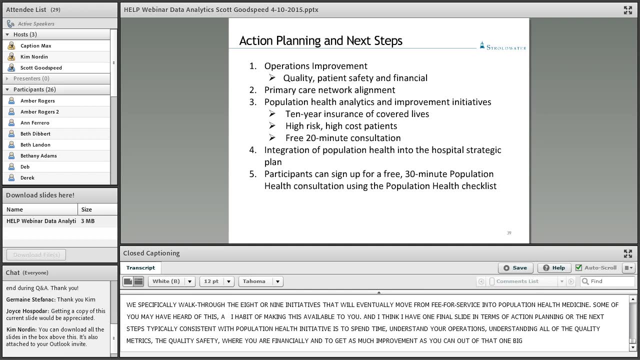 a population health initiative is to spend time- and you all do this now- understanding your operations, understanding all of the quality metrics, all the patient safety indicators, where you are financially, and to get, and to get as much improvement as you can in that one big bucket. 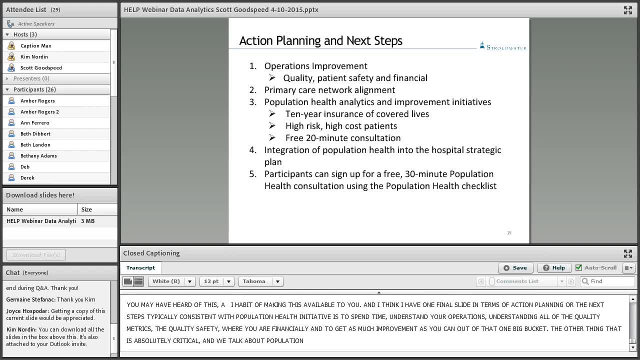 The other thing that's absolutely critical when we talk about population health is primary care network alignment. You want to make sure that you're working effectively with your primary care physicians for a lot of the reasons we talked about as it relates to population health, But they are actually the core as it relates to a population health future. 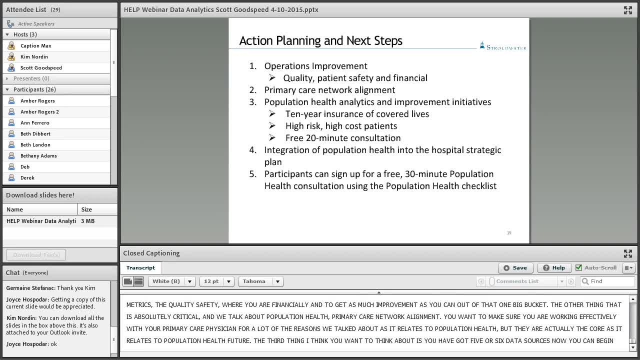 The third thing I think you want to think about is you've got five or six data sources now you can go to to begin to look at population health analytics and improvement initiatives. Again, I would try to understand what your 10-year insurance of uncovered lives are. 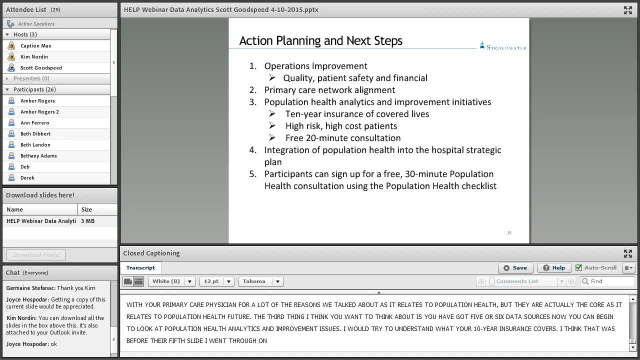 and I think that was about the fourth or fifth slide that I went through on Wednesday. So you want to understand where you are today, where those insurance covered lives will be in 2024, by payer category. You want to understand those high-risk, high-cost patients. 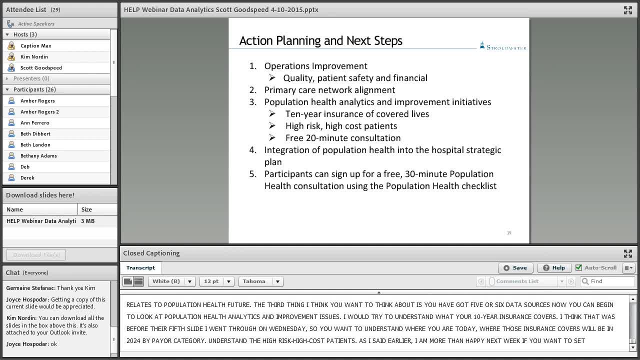 And, as I said earlier, I'm more than happy next week if you want to set up just a 20-minute consultation to look at some of your own data or talk about where you'll begin, I'm more than happy to do. Finally, the integration of your population health strategy into your hospital strategic plan. 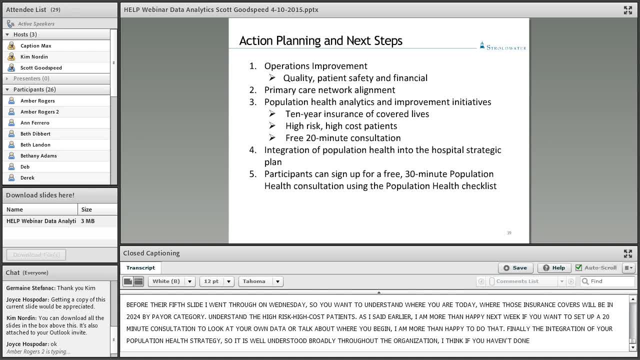 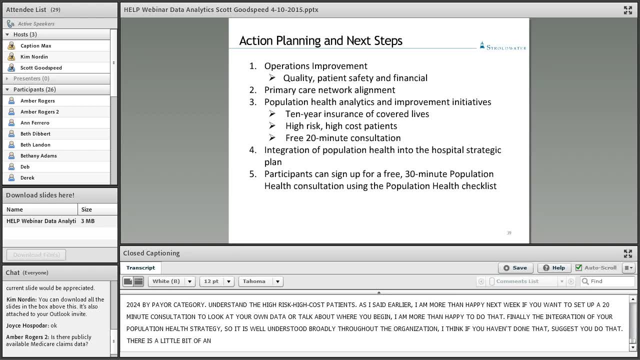 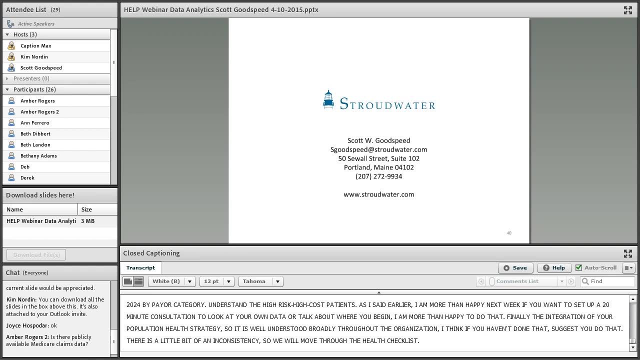 So it's well understood broadly throughout the organization. I think that's. if you haven't done that, I suggest that you do that, And you can see there's a little bit of an inconsistency here. so we'll move the kind of the health checklist consultation to 30 minutes. 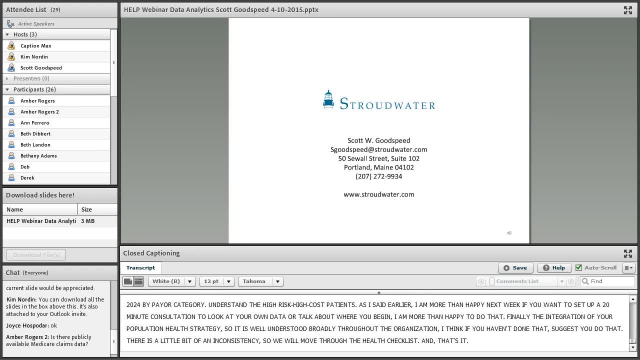 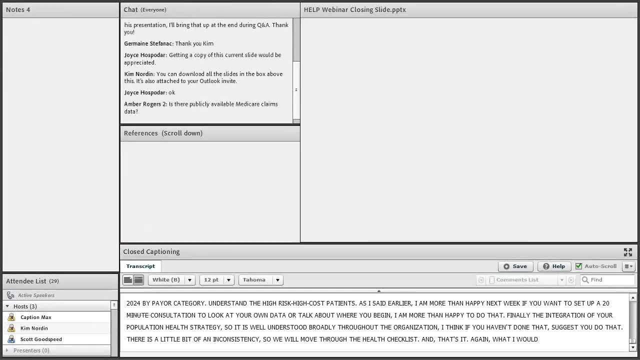 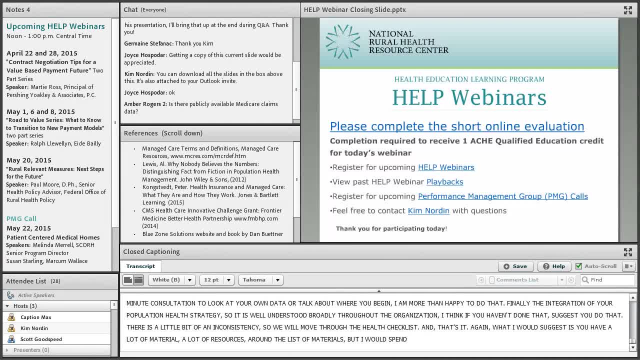 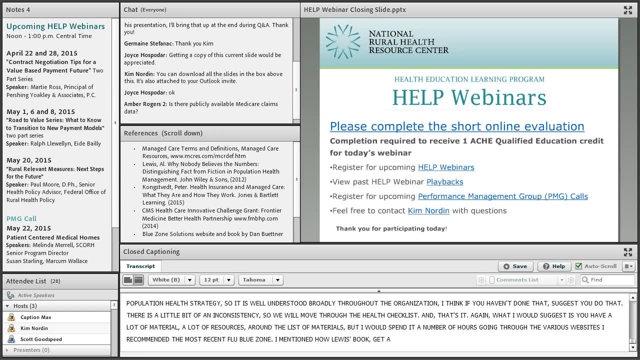 We'll send around the list of materials, But I'd spend a number of hours going to the various websites. I recommended the most recent Blue Zone books. I'd get a copy of that. I mentioned Al Lewis's book earlier And I'd at least get a copy of that for your library. 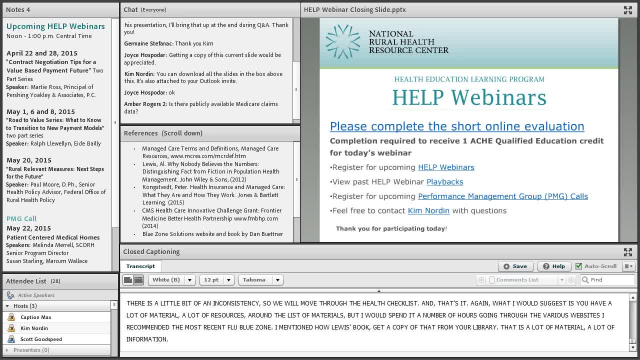 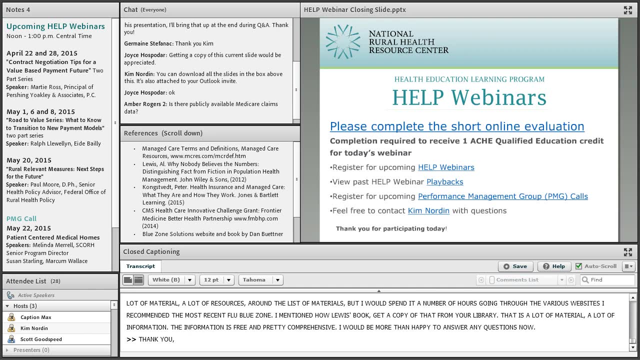 So with that, that's a lot of material, a lot of information And, again, the access to the CDC website is free and pretty comprehensive. I'm more than happy to answer any questions now. Thank you, Scott. Jermaine, was your question about service area answered? 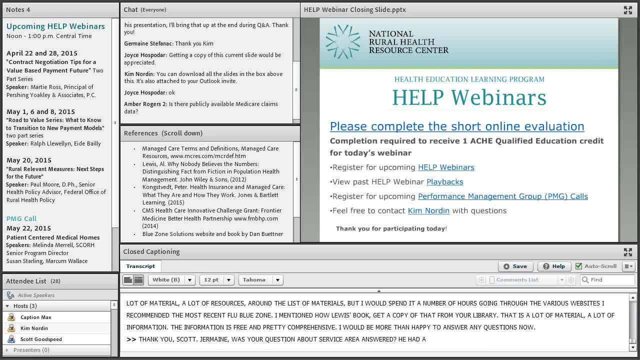 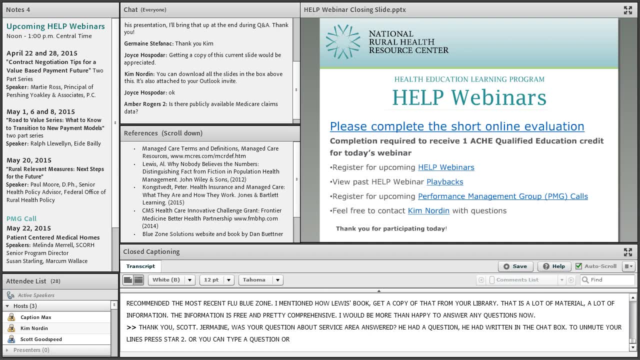 Yes, Scott Jermaine Stefanak had a question He had written in the chat box. please share service area information. To unmute your line, press star 2.. Or you can type a question or comment in the chat box. 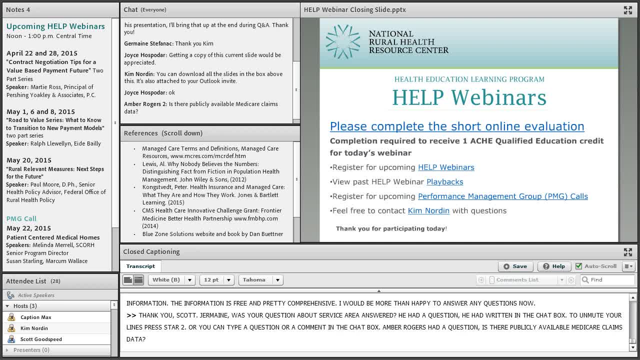 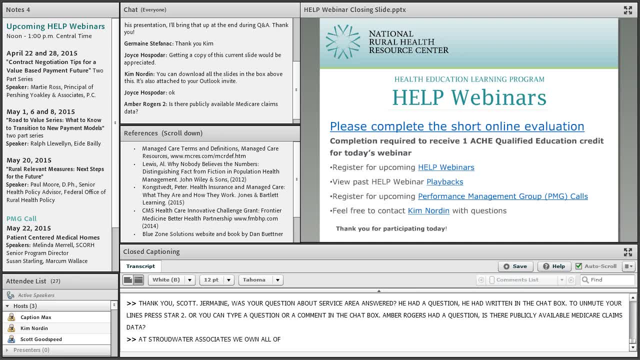 Amber Rogers had a question: Is there a publicly available? Are you available for medical care claims data? At Stroudwater we own all of the Medicare Shared Savings data. Sometimes that's available. So, for example, if you're into a federal grant which we had in Montana, all of the Medicare claims data for that innovation project was available. 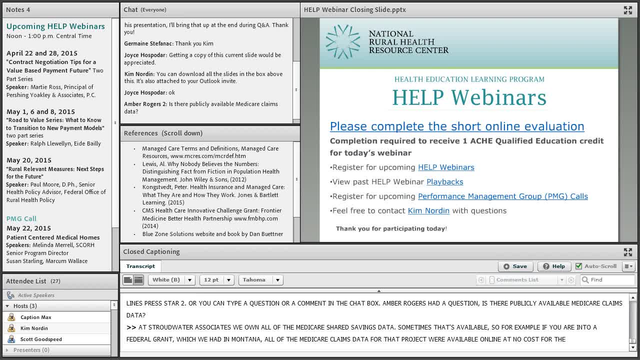 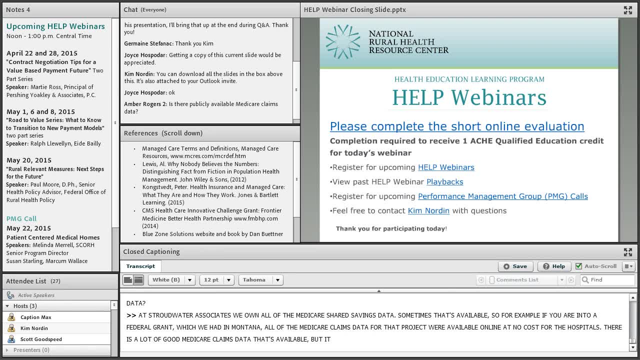 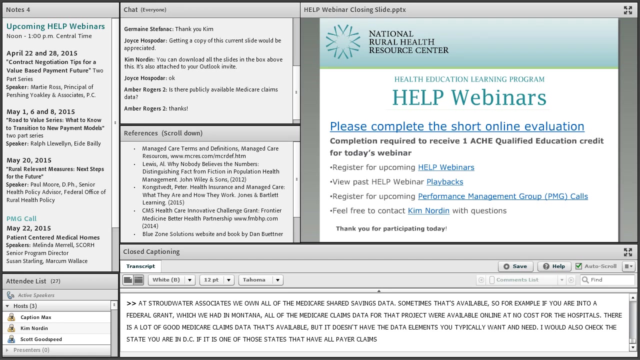 was available at no cost to those 25 critical access hospitals. There's a lot of good Medicare claims data that's available, but it doesn't have all the data elements that you typically want and need. I would also check the state that you're in to see if it's one of those states that that has all payer. 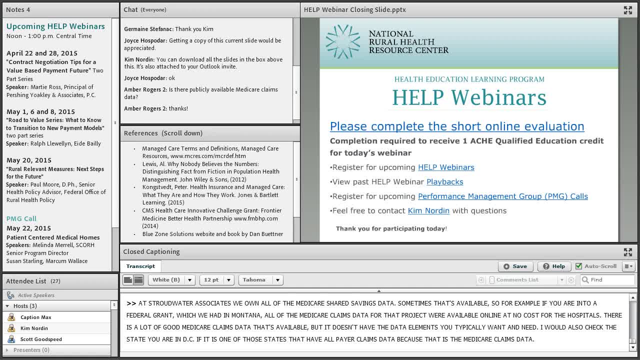 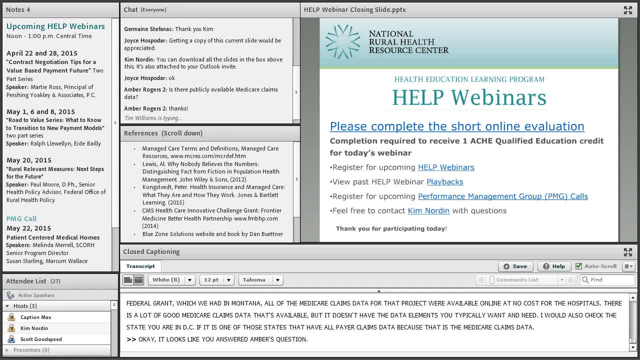 claims data, because that will also include Medicare claims data. It looks like you answered Amber's question. Does anyone else have a question? It's star 2 to unmute your line, or it looks like Tim Williams is typing a question in the chat box. 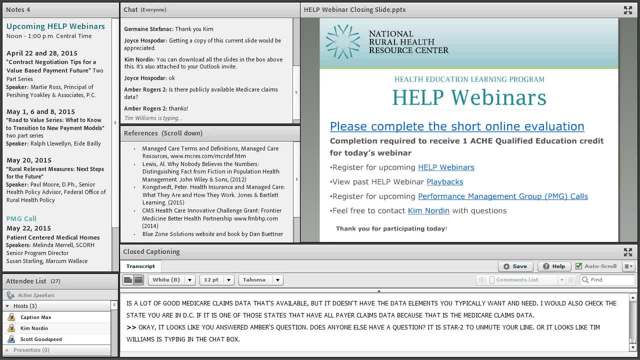 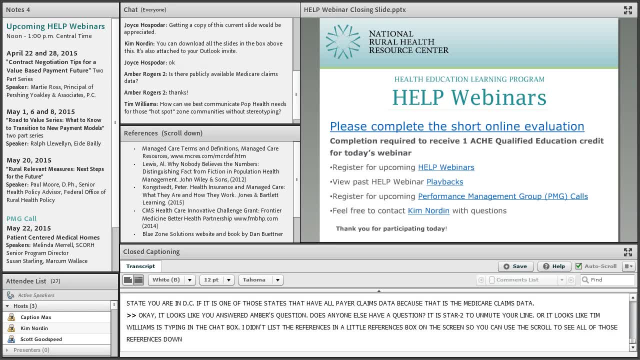 And I did list the references in the little references box on the screen so you can use the scroll to see all those references down there. Okay, I see those then that's good. Tim wants to know how can we best communicate population health needs for those hotspot zone communities without stereotyping? 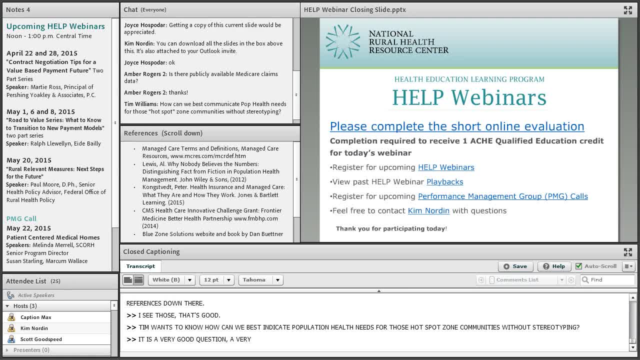 Okay, that's a good question. Tim wants to know how can we best communicate population health needs for those hotspot zone communities without stereotyping? It's a very good question. It's a very good question because if you go back to the Camden example, sometimes what they found were kind of the highest spend if 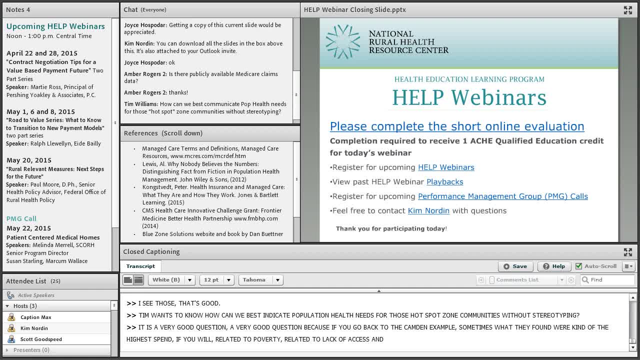 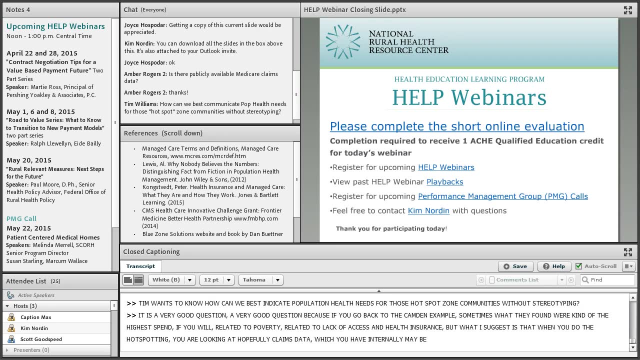 you will, related to poverty, related to lack of access and health insurance. but what I suggest is that, when you do the hotspotting, you're looking at, hopefully, claims data which you have internally, maybe publicly available claims data, as well as some of the data that's coming from the CDC. 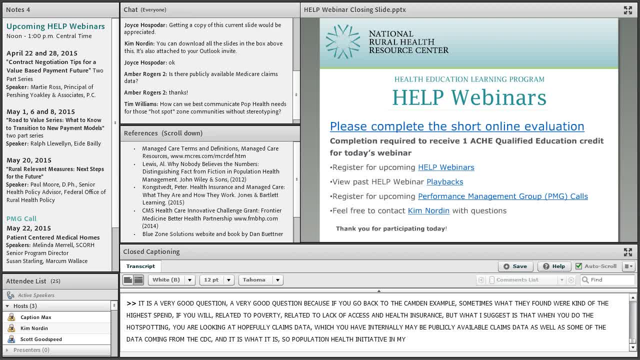 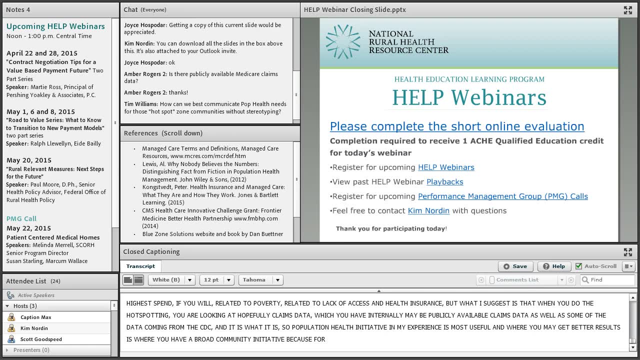 And it is what it is. So I mean to say that the population health initiative in my experience is most useful And where you may get better results. but you may not get better results- is where you have a broad community initiative, Because, for example, when we 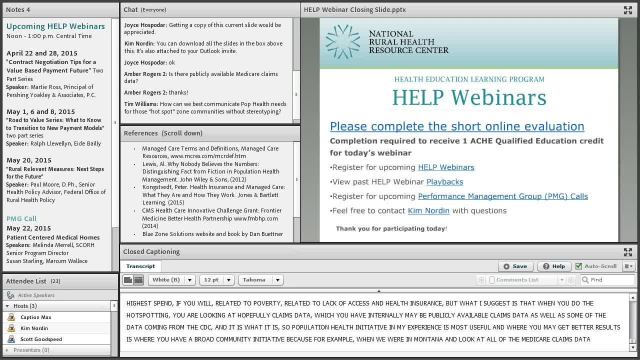 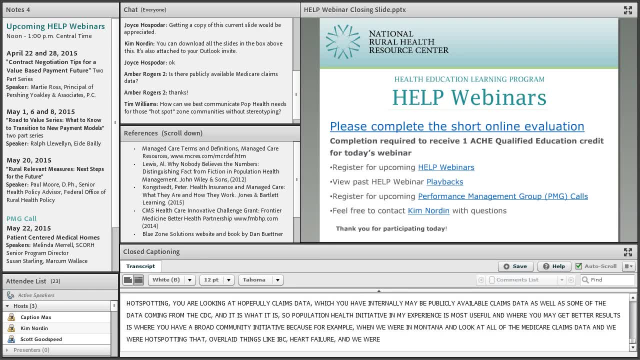 were in Montana and looked at all of the Medicare claims data and we hotspotted that. so we overlaid things like diabetes with obesity, with chronic heart failure, and we were looking at some communities, some counties, where maybe stereotyping is a good idea. and then we looked at some communities, some counties, where maybe stereotyping 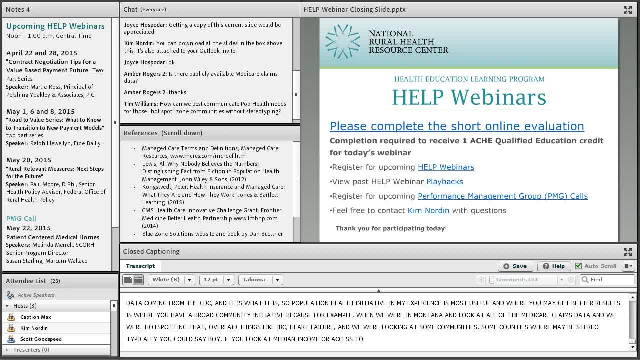 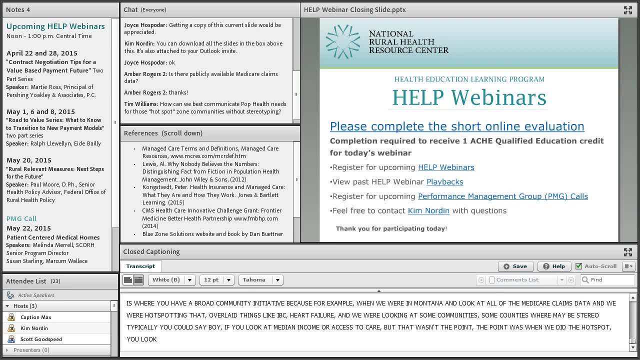 is a good idea. and then we looked at some communities, some counties where maybe stereotyping, you could say, boy, if you look at the median income or if you look at access to care. but that wasn't the point. Okay, the point was when we did the hotspot is we're looking at high cost, high risk and in fact, how do we reduce? 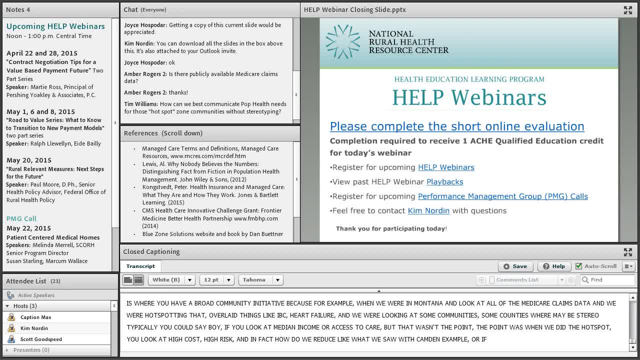 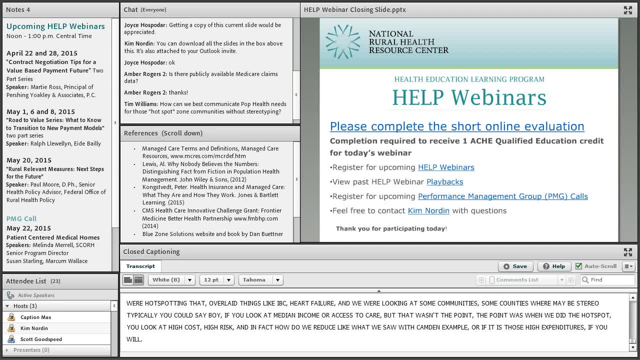 Okay, whether it's the fall rate, as we saw in the Camden example, or whether it's those high expenditures, if you will. Hi Scott, This is Bethany Hey, Bethany, Hey. at first glance, I bet there's a few small rural hospitals out there thinking, oh my goodness, with all their hats that they're wearing. 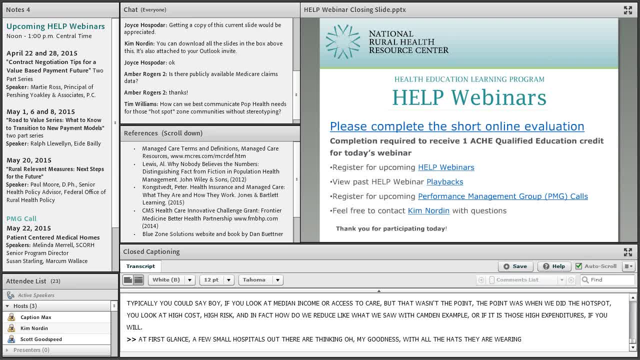 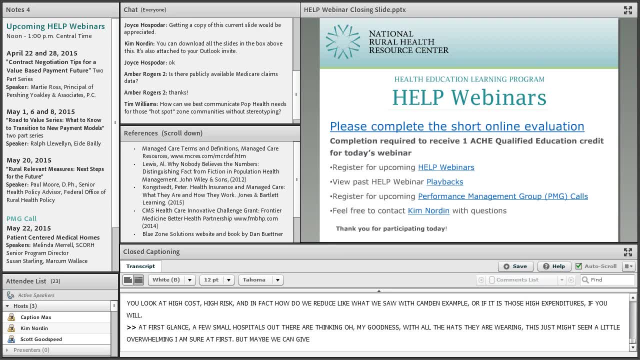 multiple hats to do all the jobs that they're doing. This just might seem a little overwhelming, I'm sure, at first, But maybe we can go to that point. But maybe we can go to that point. So I'm sorry. 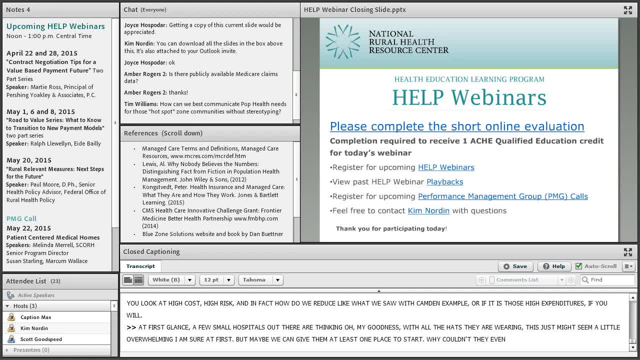 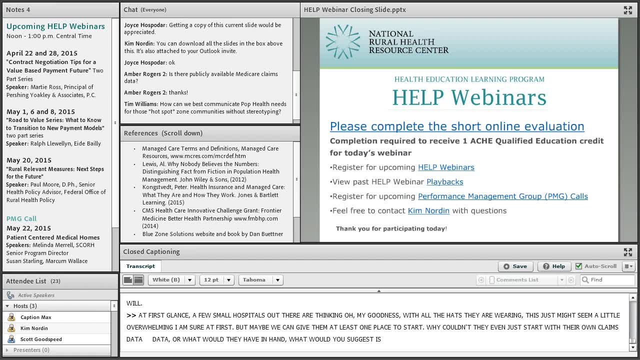 Will you go ahead, give them at least one place to start? I mean, why couldn't they just even start with their own claims data, Or what would they have in hand? What would you suggest as a simple one place to start looking at targeting that 1% or that 10% that really impacts their overall operations anyway? 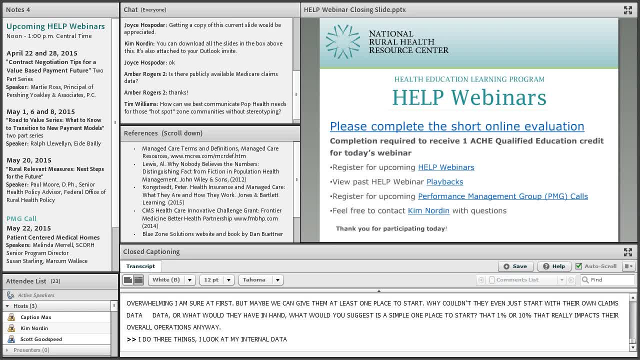 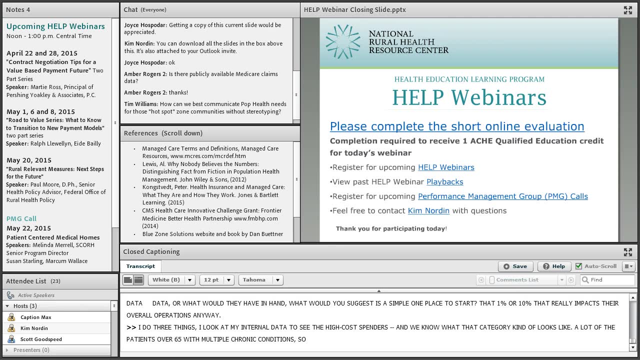 I do three things. I look at my internal data to see who the high-cost spenders are, And we know what that category is going to look like. It's going to be a lot of the patients who are over 65 with multiple chronic conditions, So I would try. 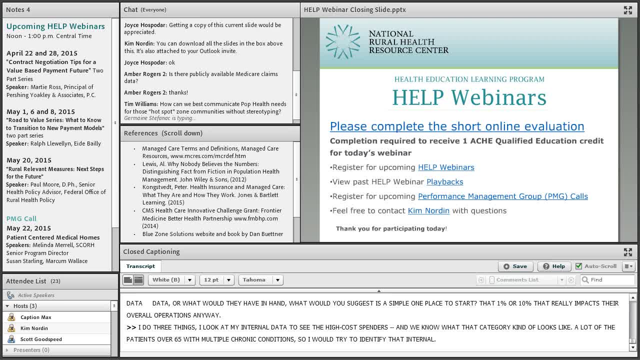 to identify that internally. The other thing, I think a simple framework, because you're not going to be able to do a lot of the work that you're doing, but you're going to be able to do a lot of the work that you're doing. 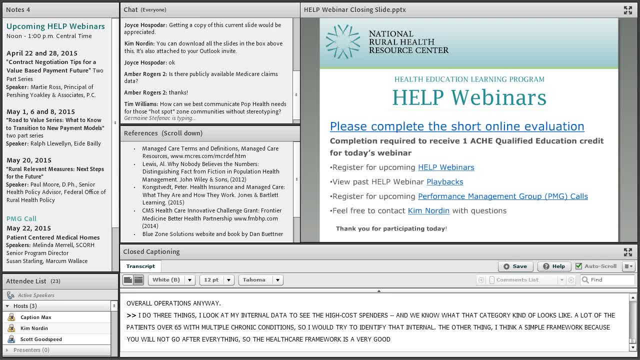 So I'm not going to go after everything. So the Mons Point Healthcare framework I think is a very good starting place And I wouldn't have any more than they've got one, two, three, four. they've got six indicators that. 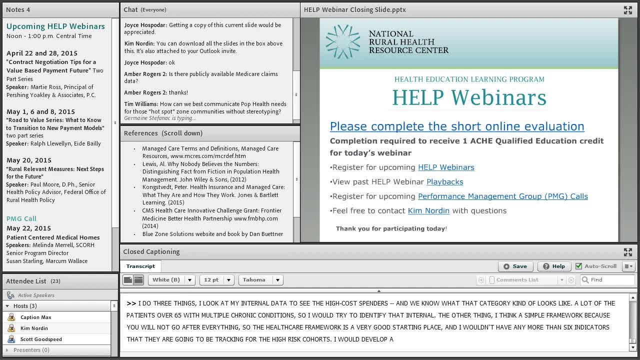 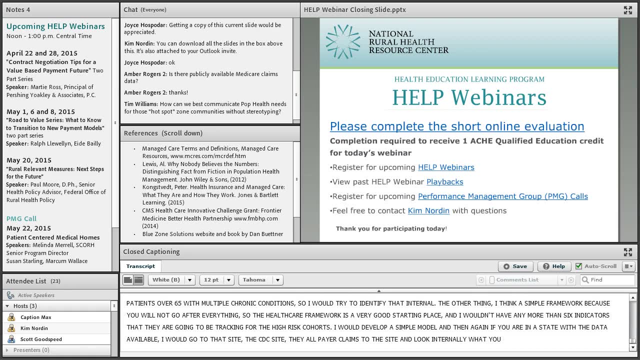 they're going to be tracking there as it relates to those high-risk cohorts. So I develop a simple model And then again, if you're in a state where you have all payer claims data that's available, I would use. I would go to that site too. So I'd go to the CDC site, I'd go to the all payer claims data site. I'd. 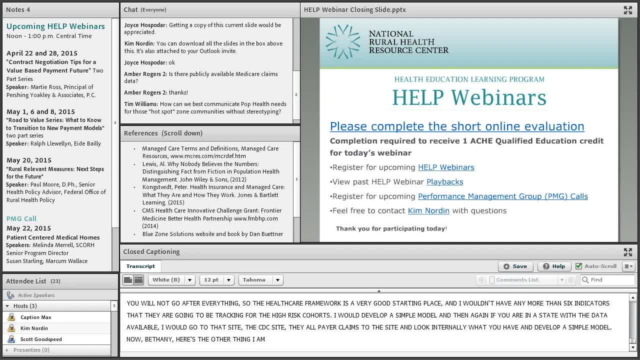 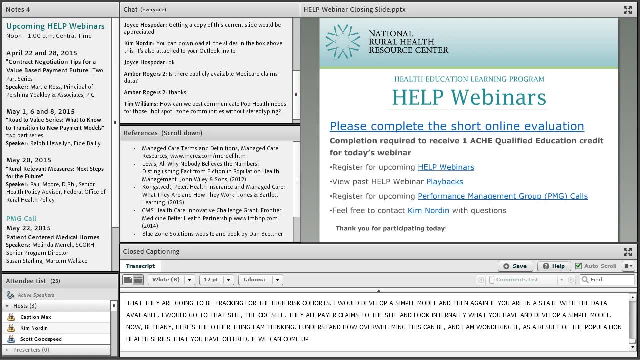 look at internally what you've got and develop a simple model. Now, Bethany, here's the other thing I'm thinking, because I understand how overwhelming this can be, And I'm wondering if, as a result of the population health series that you have offered, if we could come up with a simple 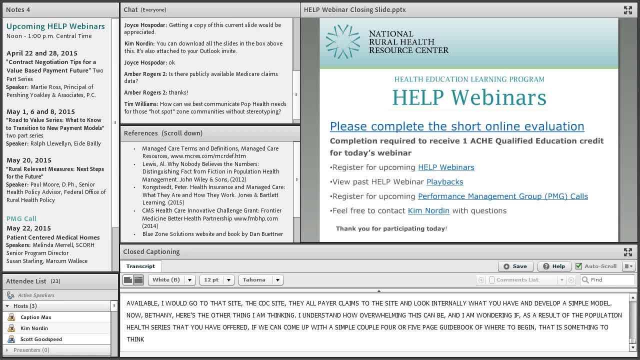 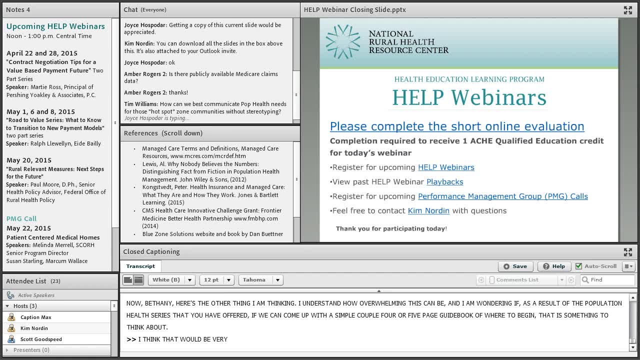 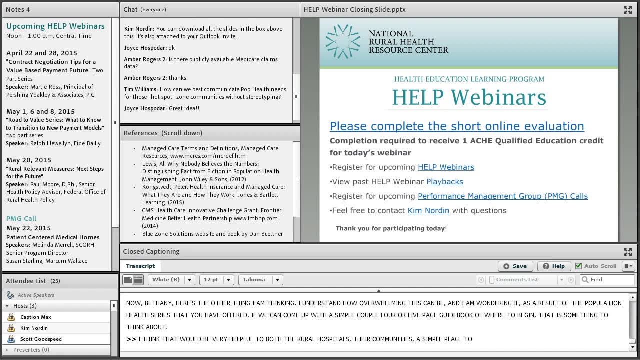 couple four or five page guide book in terms of where to begin. that's something to think about. I think that would be very helpful, beneficial to both the rural hospitals, their communities. you know, a simple place to start, something to follow: one, two, three. I think that's also. 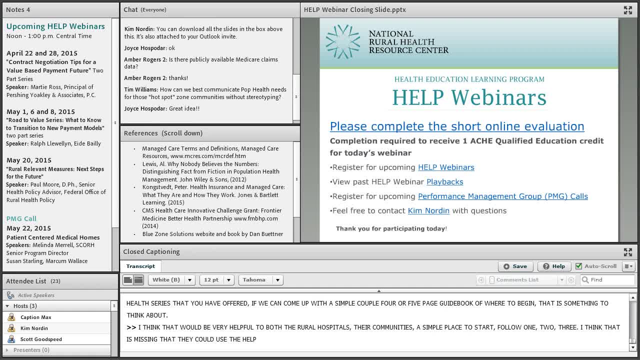 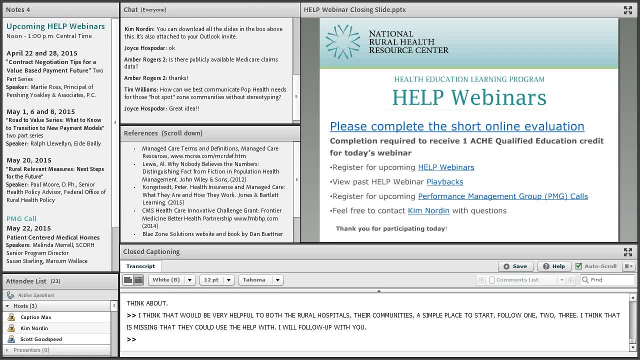 something the state offices could benefit from and they could use to help their communities, So it's a good idea. I'll follow up with you. Yeah, And I'm sorry, and I'd like to hear from the people who are on the call. 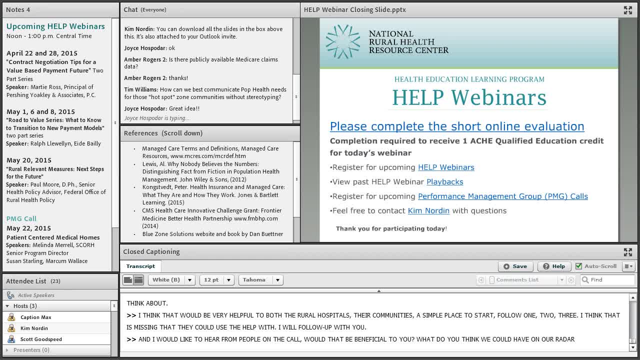 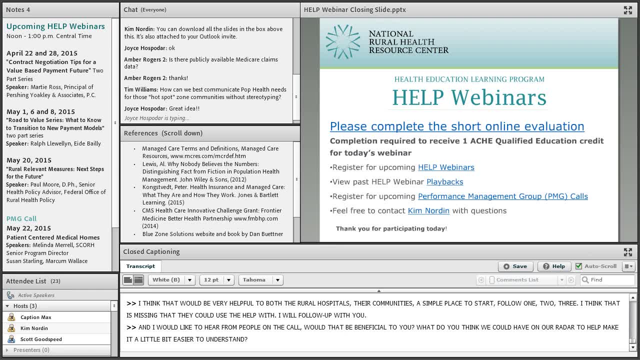 Do you think that would be beneficial to you? What do you think that we could have on our radar to help them make it a little more easier to understand step one, two, three. Sorry, So they would have typed in some of their answers or questions. That would be great, I'm sorry. Go ahead. 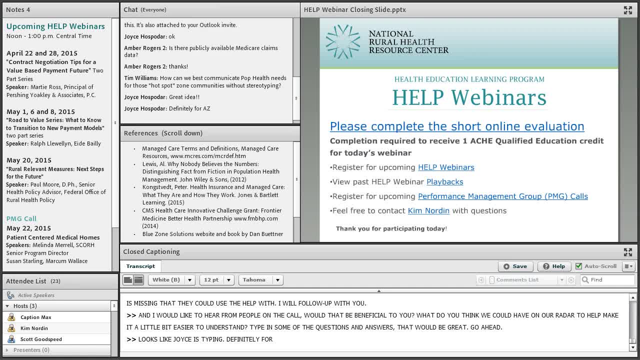 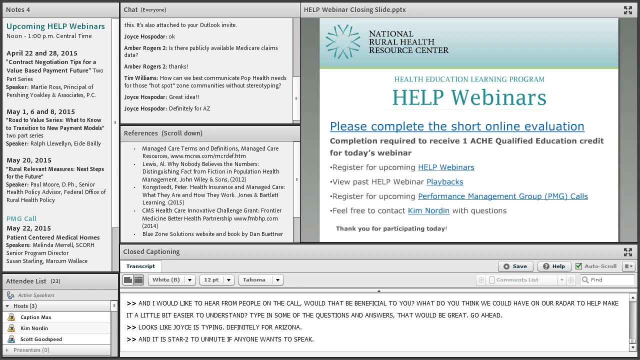 Looks like Joyce is typing Definitely for Arizona. She said, And it's star two to unmute your line if anyone wants to speak. Looks like you have a question from Tim about the hotspots. Okay, Actually, we Tim Williams. how we can best communicate pop health needs for 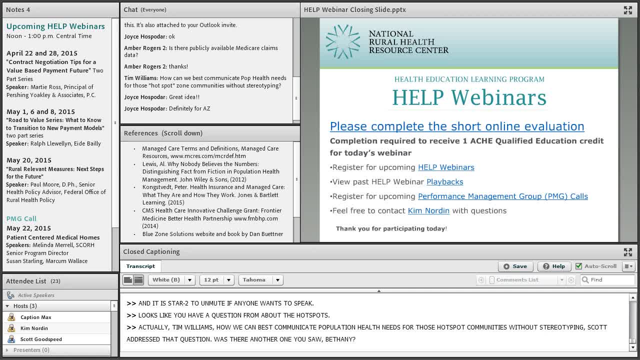 hotspot communities without stereotyping, And Scott already addressed that question. Was there another one that you saw, Bethany? Nope, Sorry about that, Just got confused, Thank you. The other thing: I'm looking at the future conferences and there's there's one. 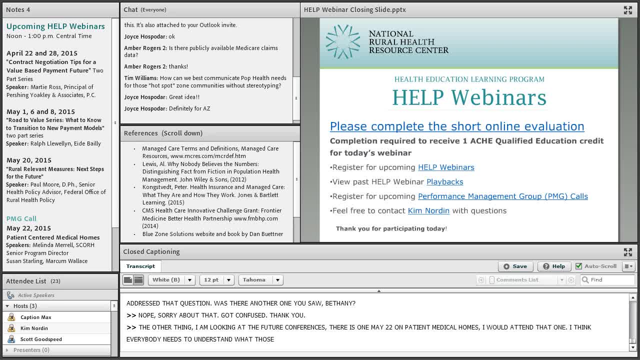 May 22nd on patient centered medical homes. I would attend that one. I think everyone needs to understand what those, what those are and their value. moving forward Great. Anymore questions? You can register for that right on our website. Great. 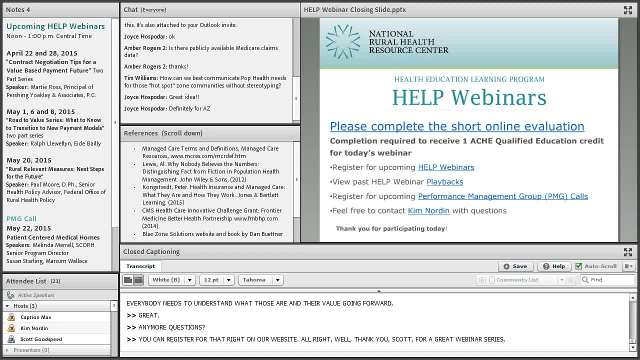 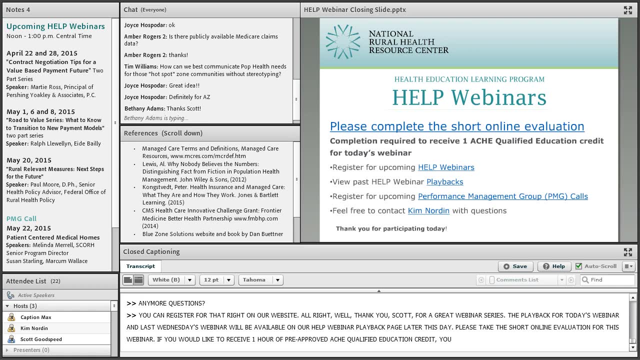 All right. Well, thank you, Scott, for a great webinar series. The playback of today's webinar and, yes, and last Wednesday's webinar will be available on our help webinar playback page. later today I'll add it. Please take the short online evaluation for this. 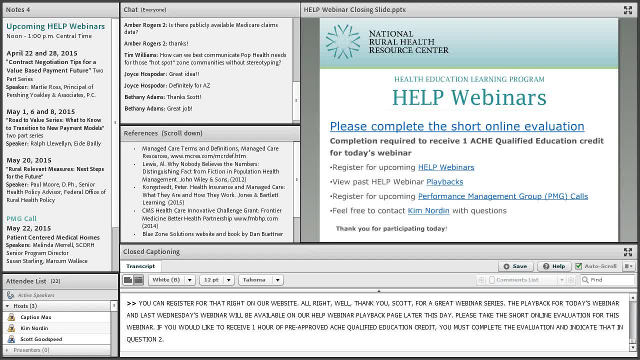 webinar. If you'd like to receive one hour of pre-approved ACHE of qualified education credit, you must complete the evaluation and indicate that in question too. To take the evaluation, please follow the link on the screen. Please join us April 22nd and 24th for our next help webinar. 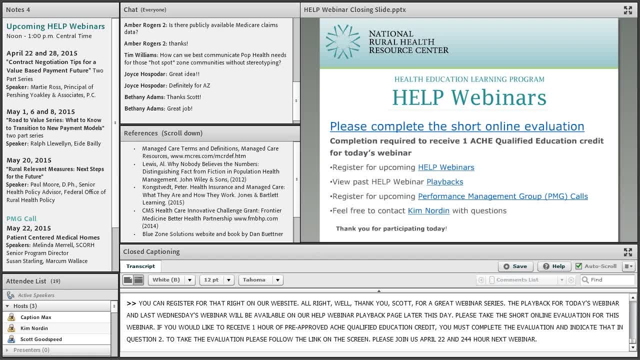 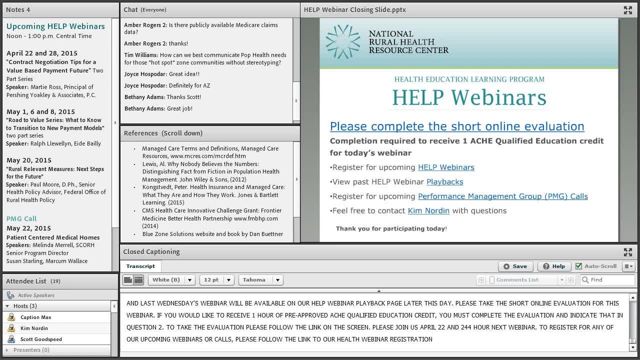 series on contract negotiation tips for a value-based payment future, featuring Marty Ross. To register for any of our upcoming webinars or PMG calls, please follow the link to our help webinar registration page. If you have any questions or comments, please contact me at.